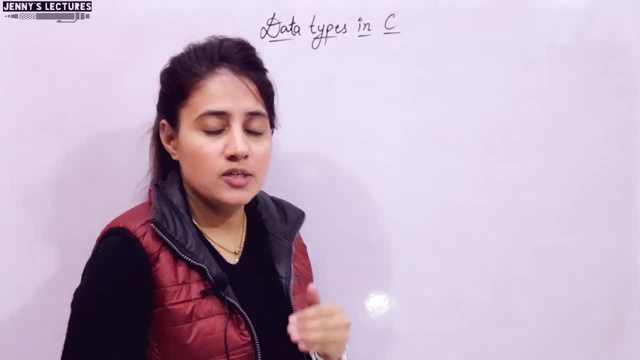 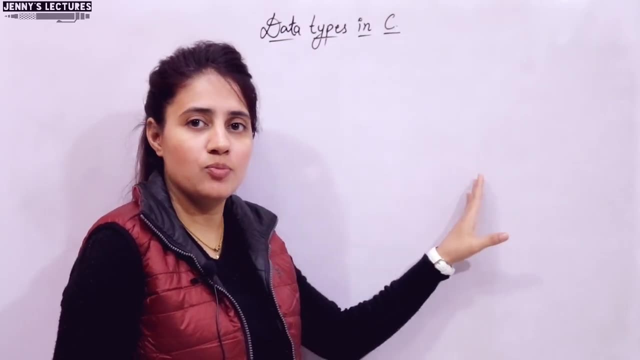 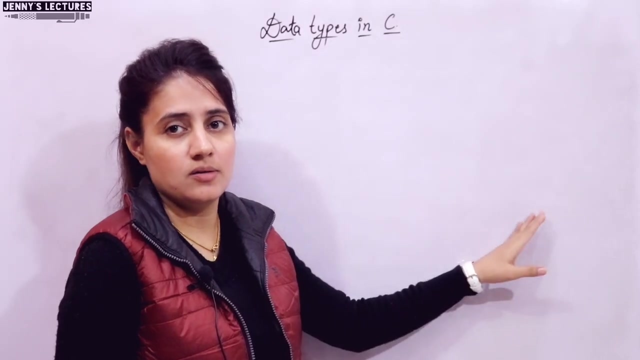 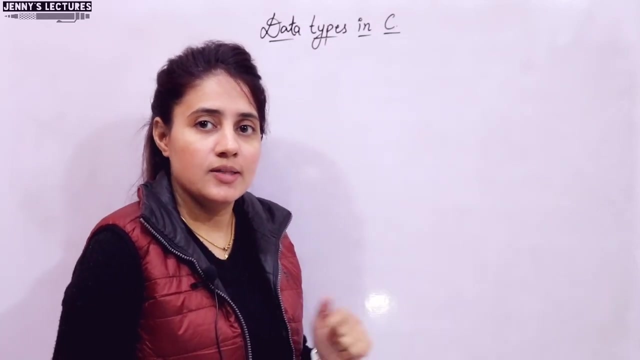 So that today- that is why I am making this video- We will discuss in this video that thing. I will give you some examples- also proper example I will take, and then we will discuss the output of that example, that line Like why you are taking different answer from that initialization, from the value you have initialized in your program, Why you are getting different answer. right, That we will discuss in this video. So, and this video is brought to you by an academy because 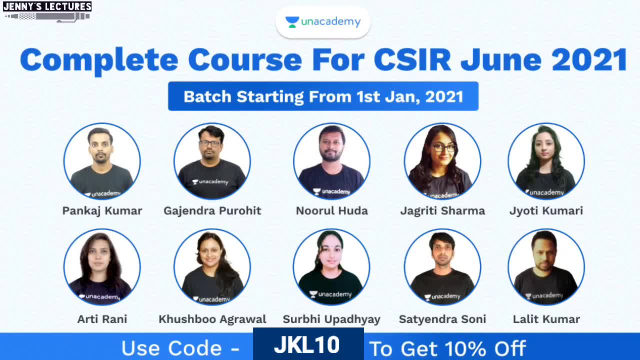 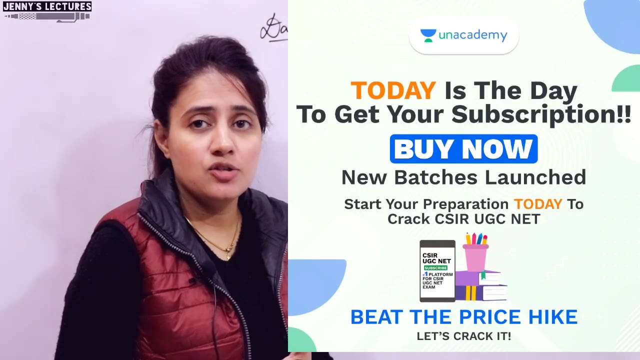 an academy has launched new batches for the aspirants preparing for CSIR UGC net June 2021.. You will get here the complete course for CSIR net exam for June 2021 exam right And these batches are like they will teach here all the subject, like life science, chemical science and mathematical science, And these batches are both in Hindi and English. So if you are comfortable in Hindi, you can watch those videos. If you are comfortable in English, you can watch those videos. 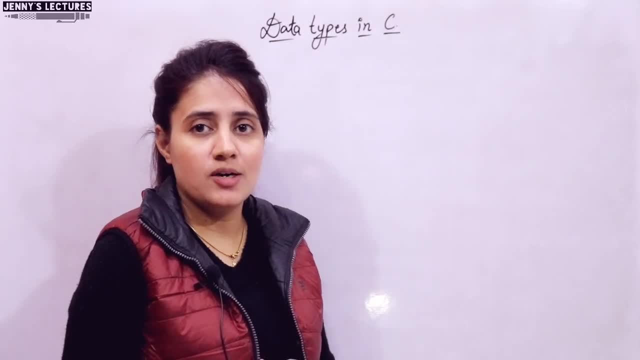 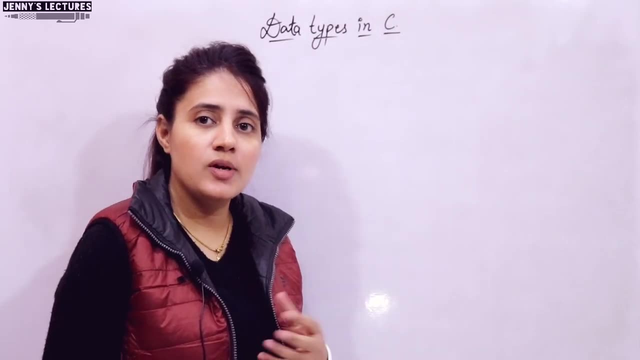 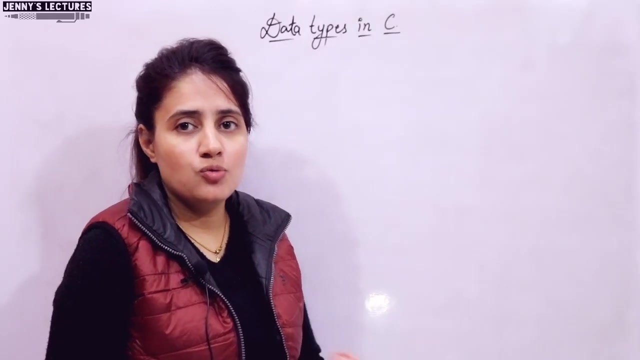 So you have the facility to choose your favorite teacher and you can watch, you can attend their classes, right. And this is what it's- a paid subscription, because you will get complete structured course for your CSIR net exam, But if you will use code, you will get 10% discount on your paid subscription, right? So if you are planning to appear for June 2021 exam, then it's better to start your preparation early. 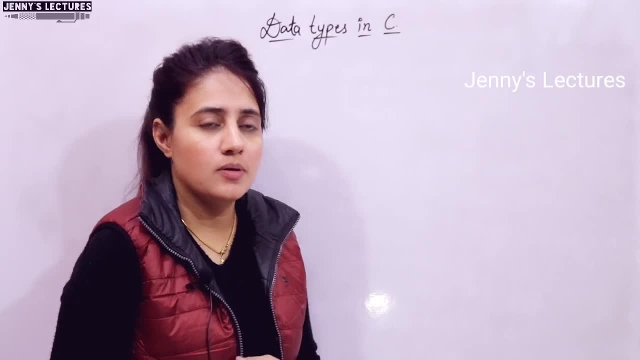 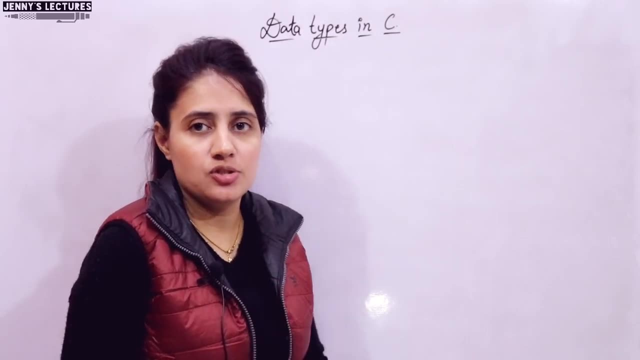 academy are going to teach you and the batch may be in hindi language, like the classes would be conducted in hindi language and they'll also provide you notes. but the notes they'll provide you, that would be in english language only. so if you are interested, you can go for it. you just have. 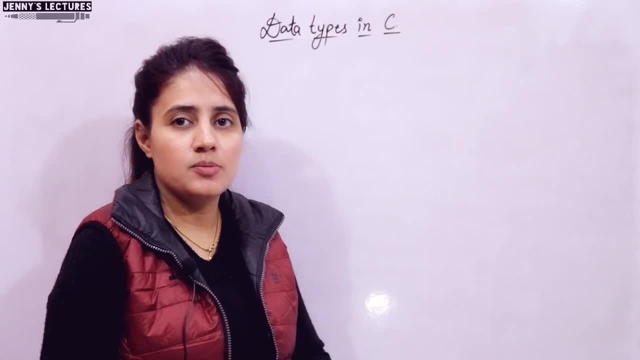 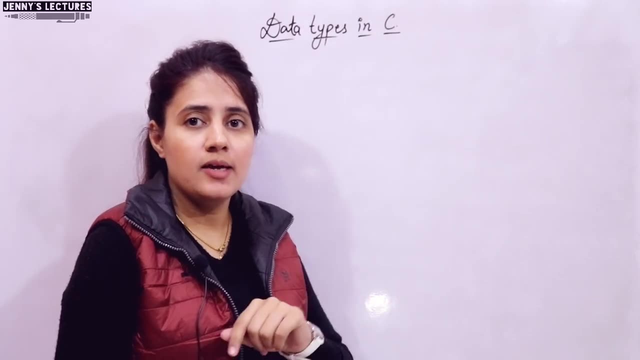 to download an academy app and you just have to get the subscription of the batch you want. they'll show you the detail, right, so i'll provide you all the details and the link, as well as the referral code, in the description box of this video. you can go and check out. so now let us continue our 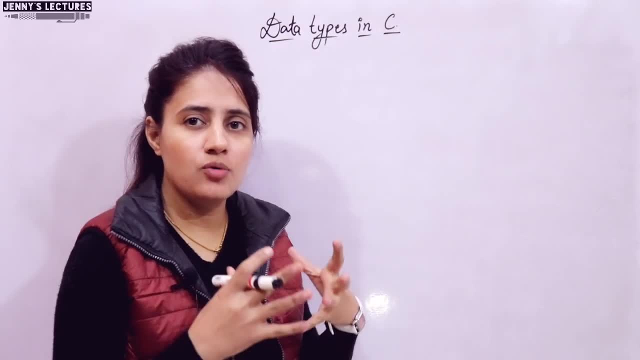 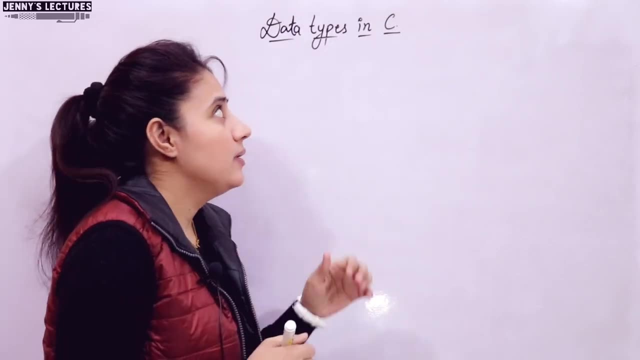 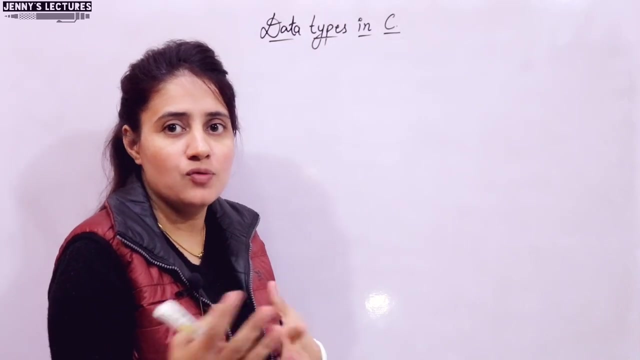 discussion on data types in c. in this video i'm going to discuss about int with proper example and some diagrammatic representation also. see i'm see in the context of 16-bit compiler. see my system on my system, if i find, if i find the size of the int, that gives me two bytes right, maybe in. 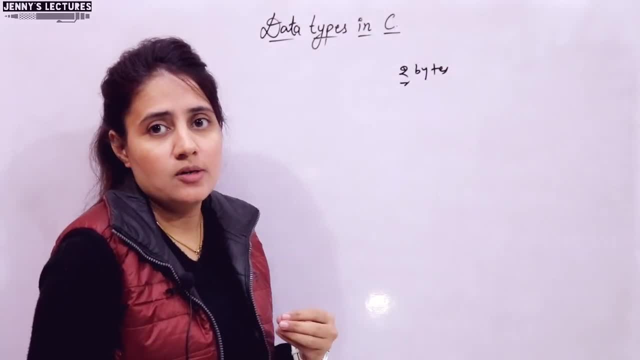 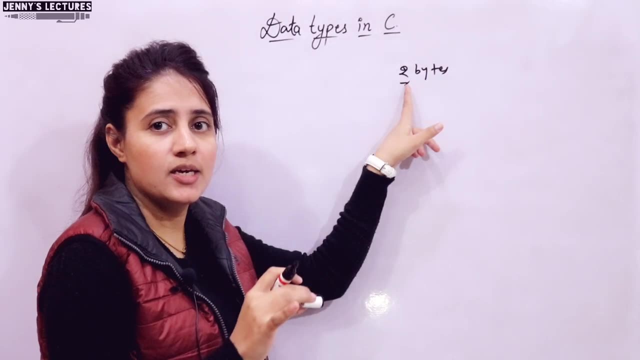 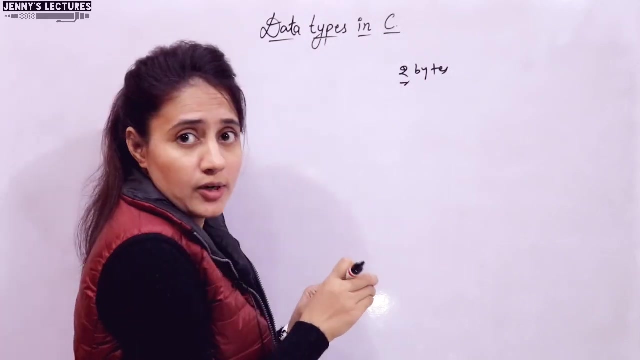 your system. if you find the size of int, it will give you four bytes you. so i'm discussing this, the lecture in the context of the two bytes. like the int is taking two bytes memory, right and long, and long is taking four bytes of memory right and short, int also taking somewhere it's it will take one byte and in on some machine it will take two bytes. now why the range of integer is lies between this: for signed int the range is this one. for unsigned it it is between this one. see for integer, suppose i'm taking two bytes. for storage integer will take two byte. so one byte means eight bits. 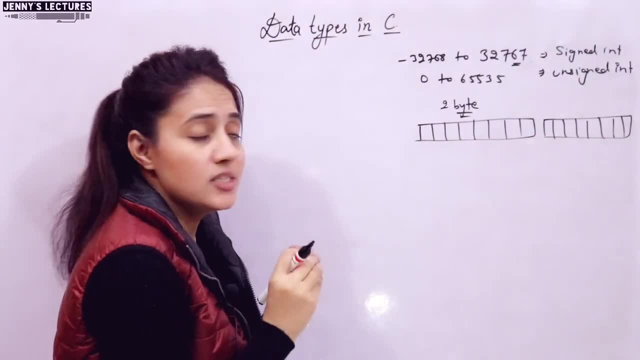 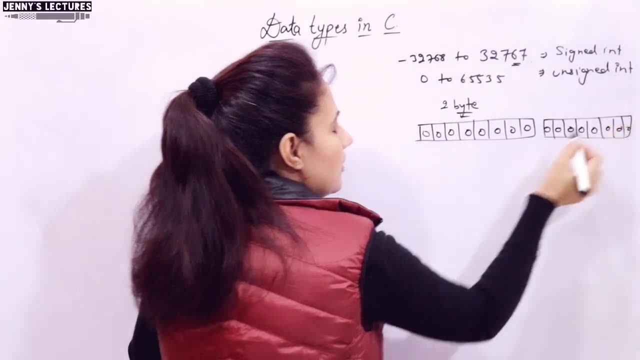 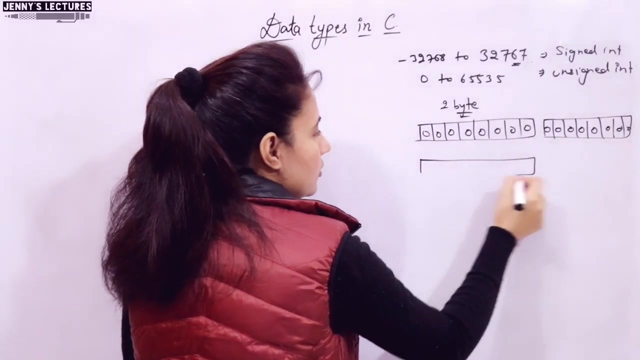 these are two. bytes means eight bits and eight bits, so the lowest number can be zero, like i am putting zero in every bit, right, and the highest number can be because binary. uh, the, the computer understand the language of zeros and ones. so we store everything in form of zeros and ones. so 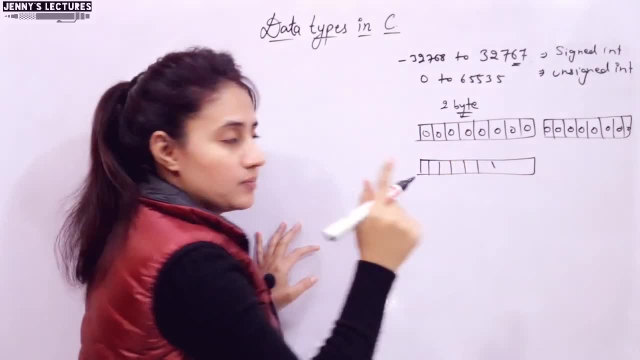 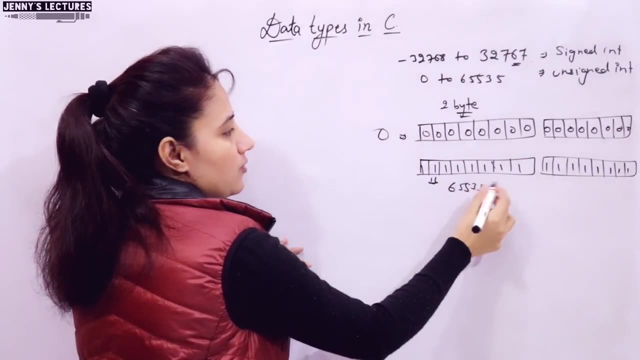 highest number can be in every cell. we can put one, so this is the highest number. so this is corresponding to zero and this number will be six, five, five, three, five. you can find out this number, the number system, when we'll discuss number system. then we'll discuss how to convert a decimal number. 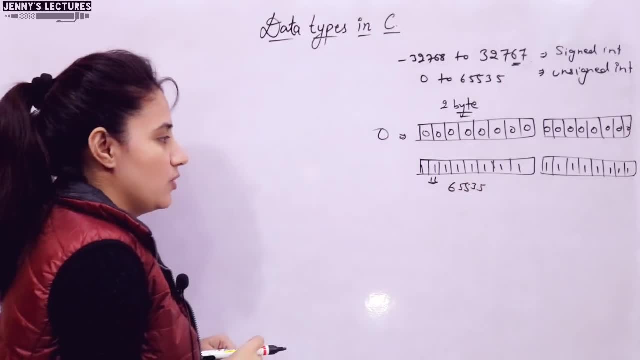 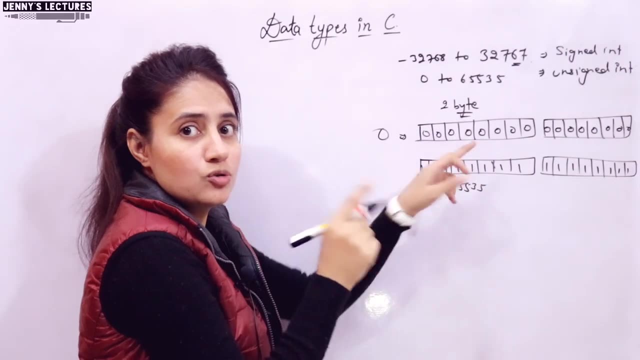 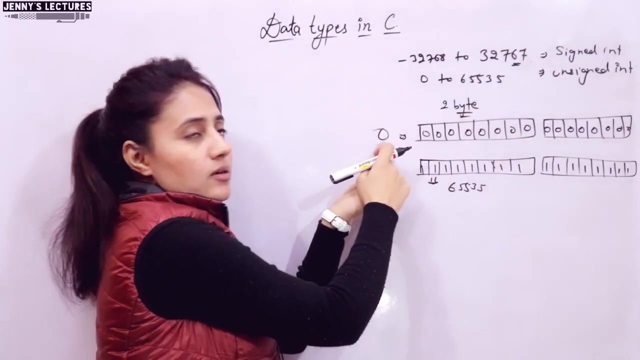 or integer into, uh, that binary language zeros and one forms. so that is why the range is from zero to this one, because the size of integer is two bytes. so within these, those using those two bytes, the, we cannot store a number in unsigned int less than zero and greater than this one. but if it comes to 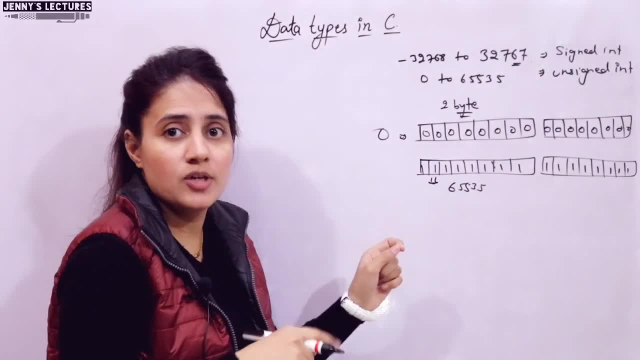 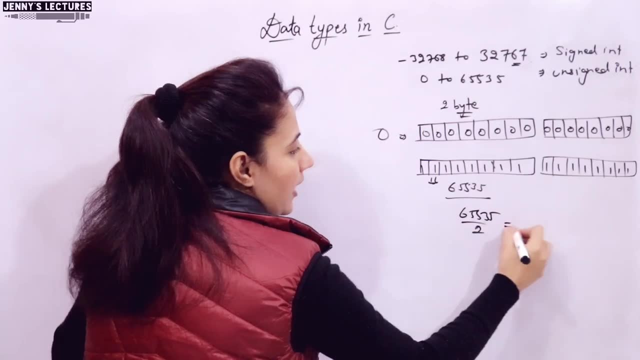 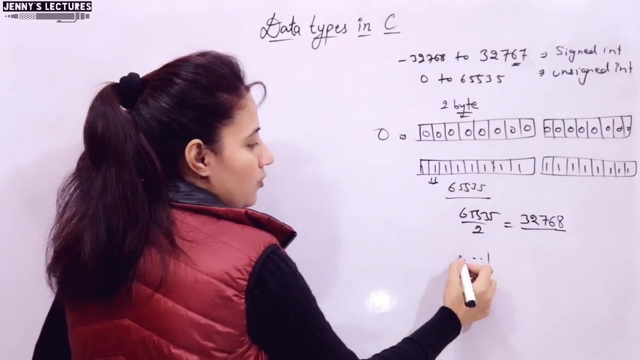 signed integer means we can store positive value as well as negative value, right? so if you divide this by two, then that would be this number, the round off number, it would be this one. so from zero to negative we have, we will take minus one, minus two and up to minus three, two, seven, six. 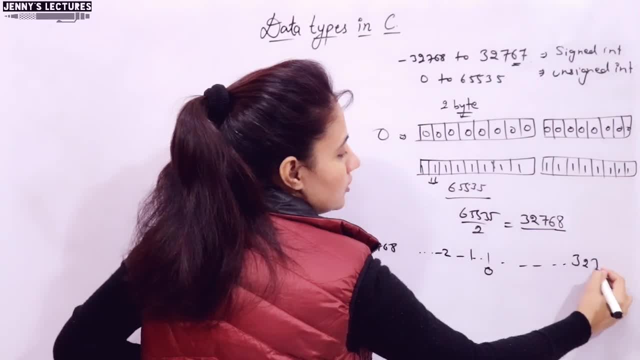 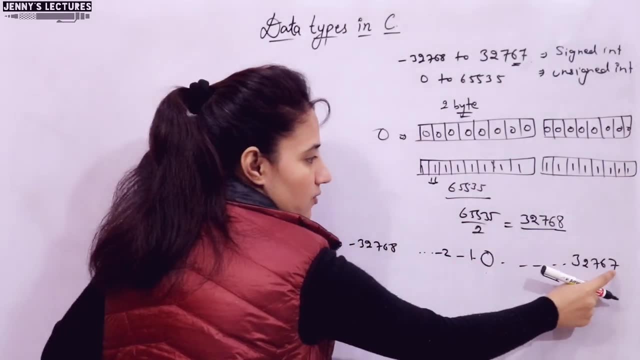 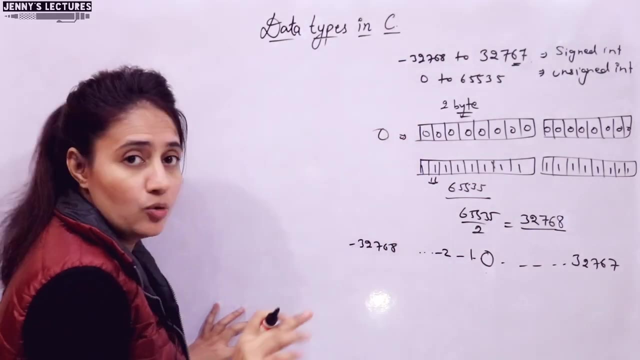 eight. but this side the range is three, two, seven, six, seven. why? because we are also including zero in positive integers. that is why this side we have till six, seven and this side we have till six, eight. that is why the range is this one: because of the size. i hope you got my point right. now let me 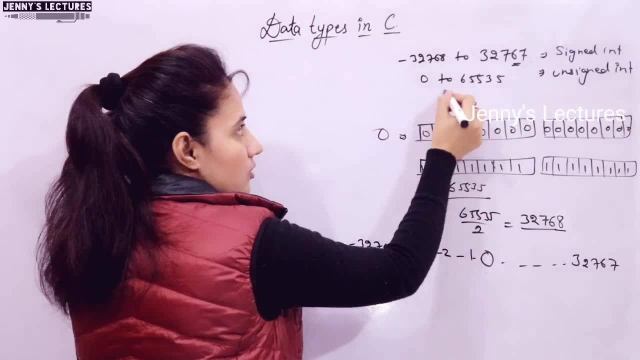 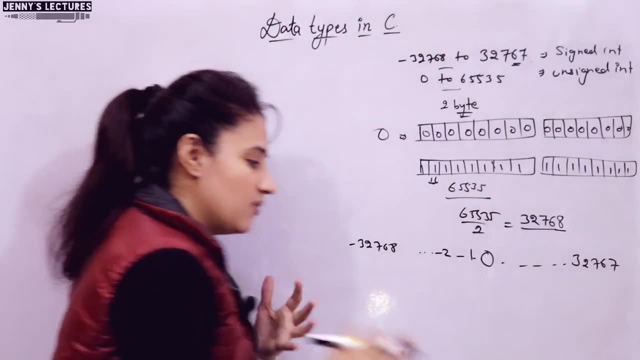 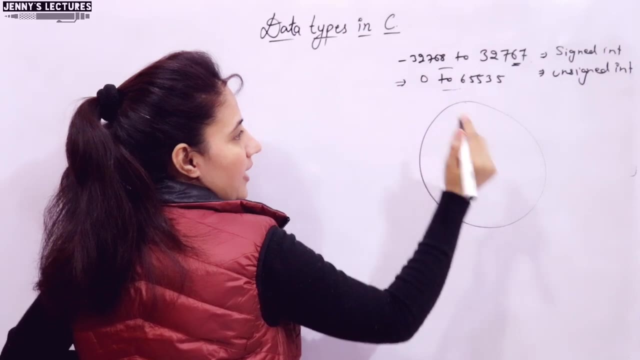 discuss it with the program and if i represent this range, this one and this one in a circular form, will represent it in a circular form. then you will get a better understanding why you are getting different answer from the value you have initialized in your program. right, suppose i'm taking this one for unsigned int, for unsigned int. that that format. 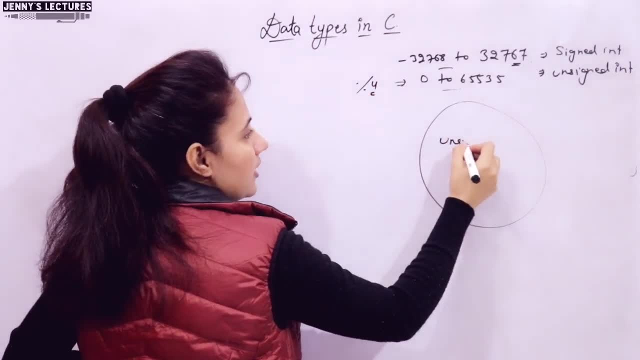 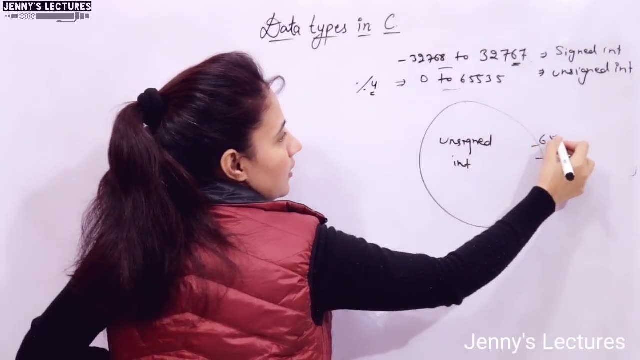 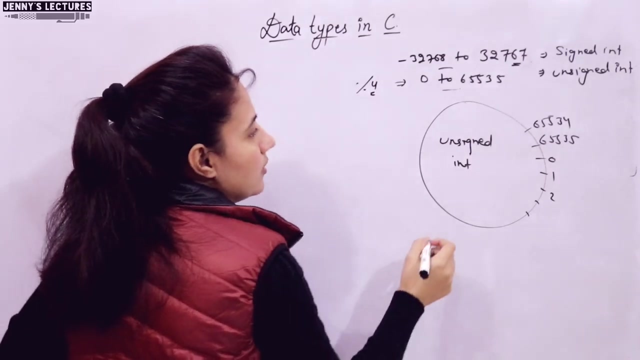 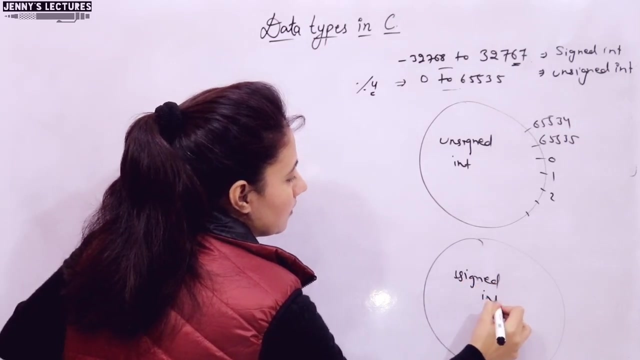 specifier is percentage u. this is for unsigned int. i'm representing it unsigned in. so from zero to zero, one, two and till six, five, five, three, five, right, six, five, five, three, four. this one, right now. next one is suppose i'm representing it, this circle for signed int. so from zero. 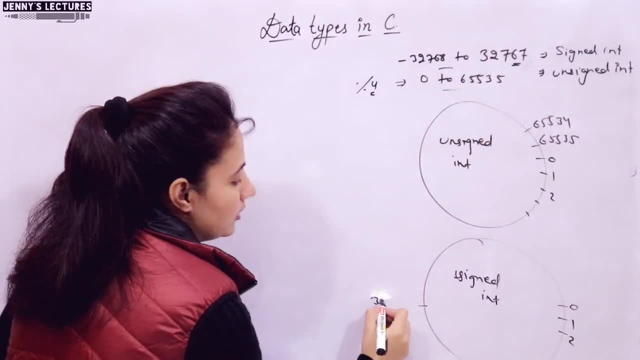 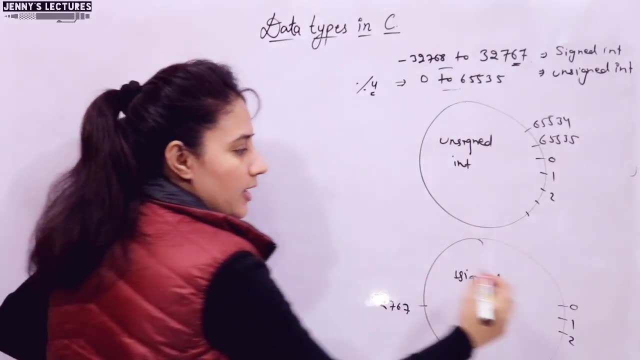 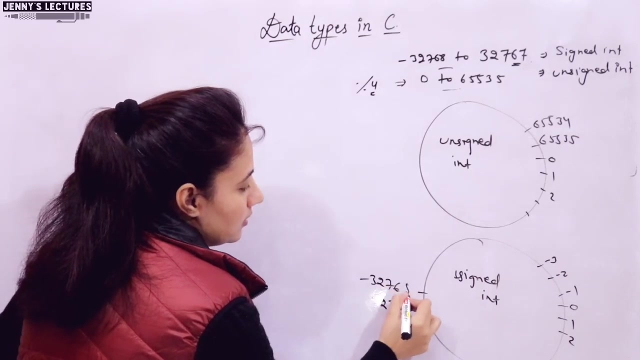 to one value would be. the positive value would be till three, two, seven, six, seven. this side i'm taking positive values and this anti-clockwise i'm taking negative values. so minus one, minus two, minus three and so on, and here you will get minus three, two, seven, six, eight. here we will have 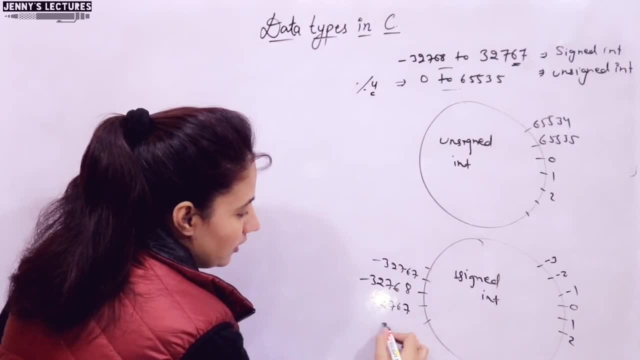 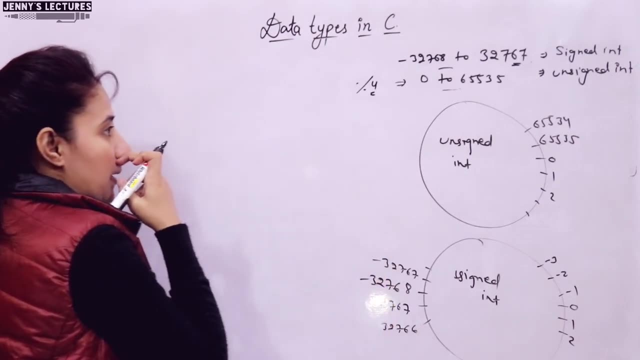 minus three, two, seven, six and so on. Here we will have 3,, 2,, 7,, 6,, 6.. I hope you are getting the circle. Now let us take one example and assign some values to integer. Suppose I am adding this, a simple program. 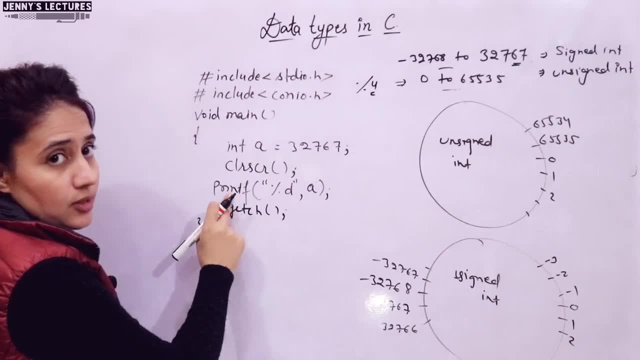 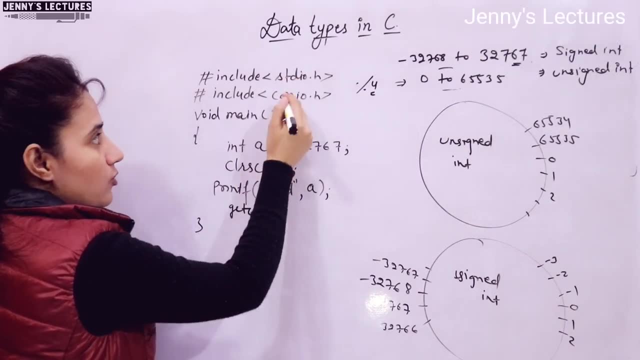 Why you are including stdih- Because I am using printf here- The definition, you can say, the declaration, the meaning of this is where In this library. And why you are including conuh console input output Because of this function: getsh and clrsr. This is for. 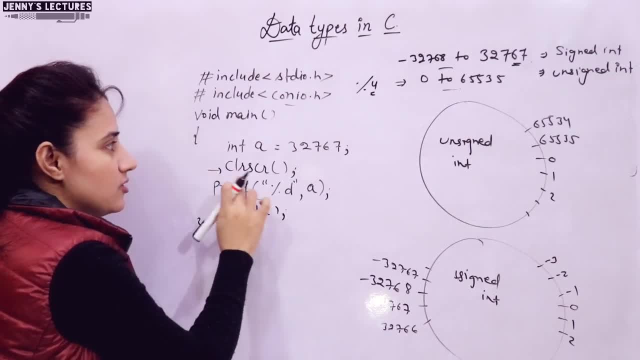 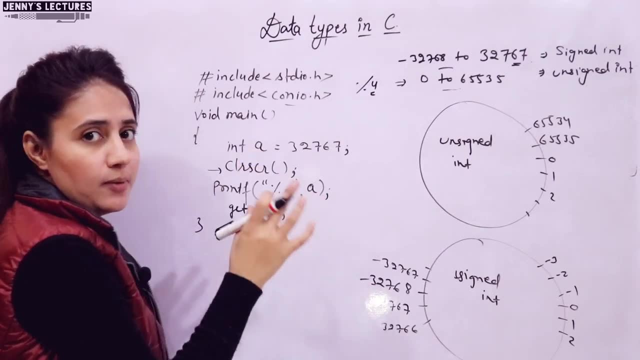 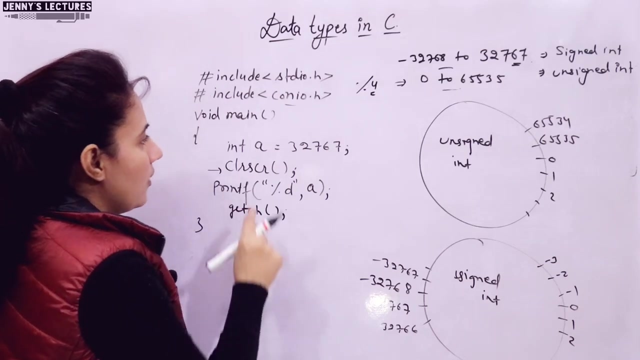 clear screen, And always in C we use clear screen function. after the declaration of the variables: Here we are declaring a variable and initializing the variable in the same statement, So after that we will write clrsr. If you write before this, you will get an error. So now I am going to put a. 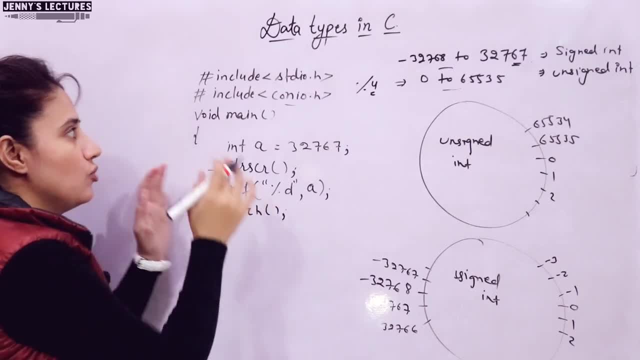 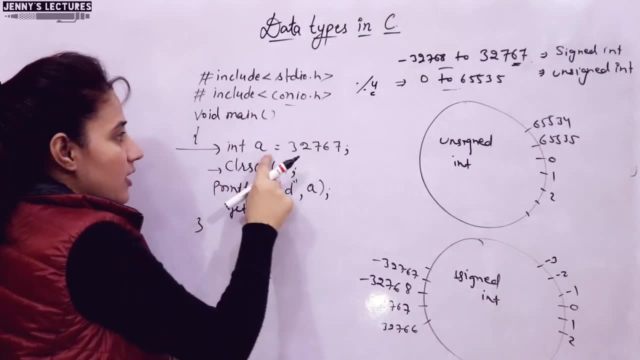 value. See first of all the control will go. when you execute this program The control will go first of all the first line within the main function. Always, execution would be started from main function. First line is int. a is equal to this one. It means I am declaring a variable, So in memory a space would be allocated to 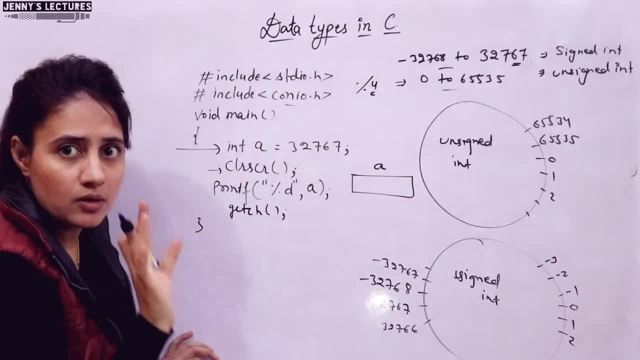 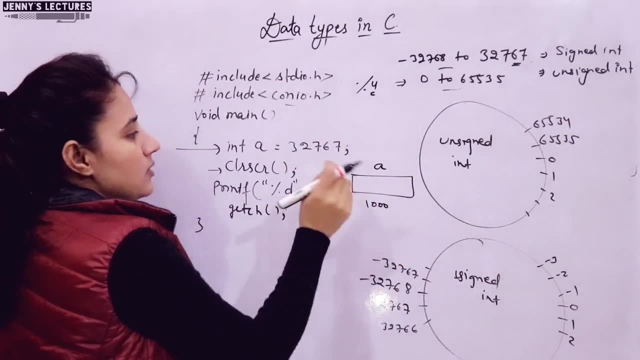 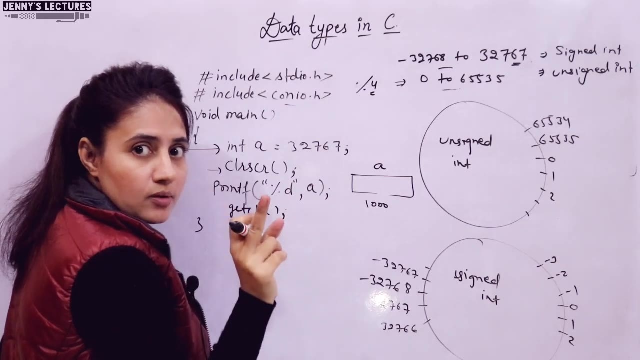 this one, And the name of that location is a Variable- is named memory location. Suppose location is I don't know address, is suppose 1000.. Right, Now, we have to put something here. Now we are initializing this one. I want to put this value here. Right, This is what int is. 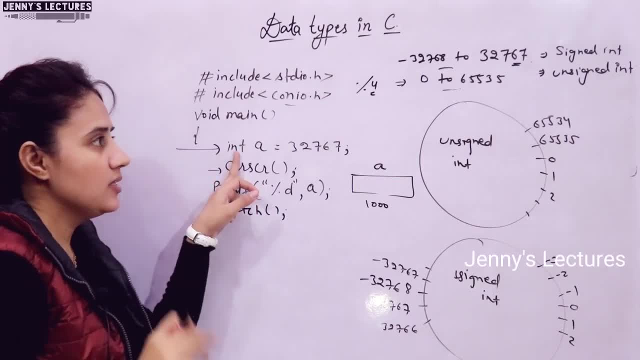 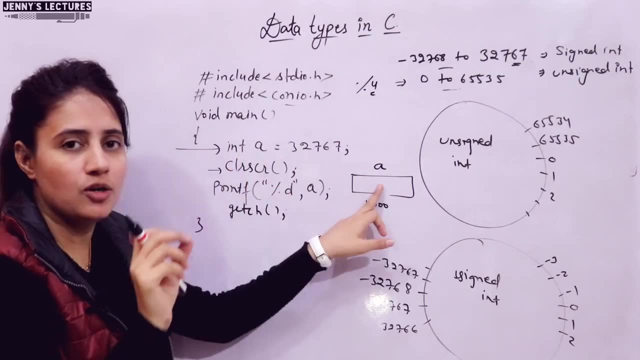 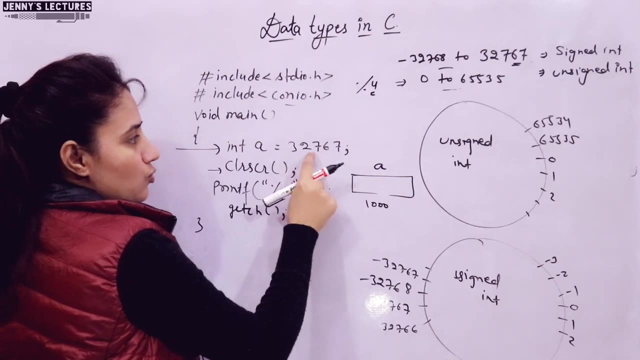 So now, see it is, if I am not writing signed or unsigned int, then by default it is signed integer. We can store positive value as well as negative value within this box, within in this memory, Right? So now it is signed one, So go for this one. 32767.. Within this circle, do you have? 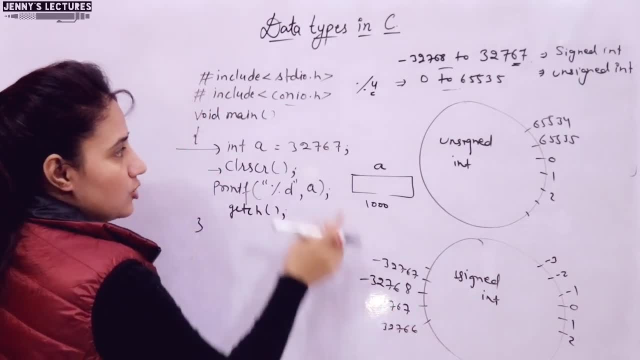 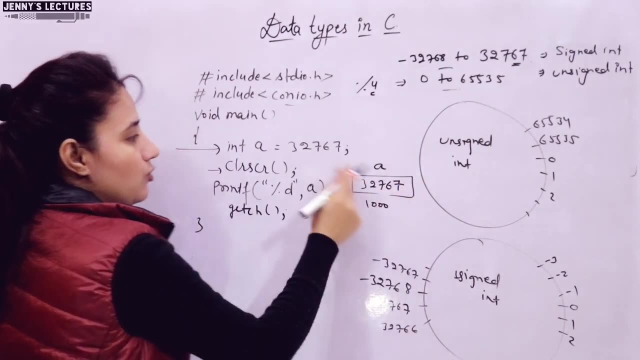 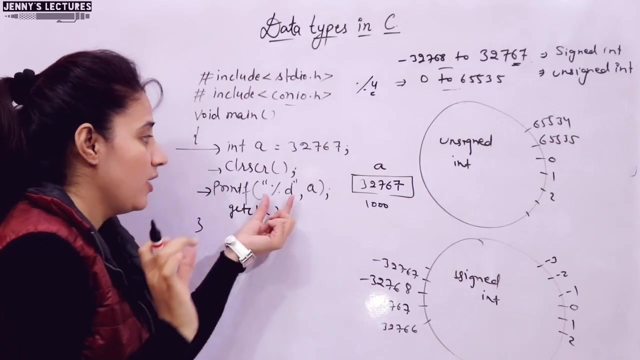 this number. Yes, I have 32767 the range, So this number is within this range, Right? So 32767. it would be stored in memory And then when you will print this value- printf- %d- %d- format specifier- This is going to play a very important role, Right? You will get to know in this video. 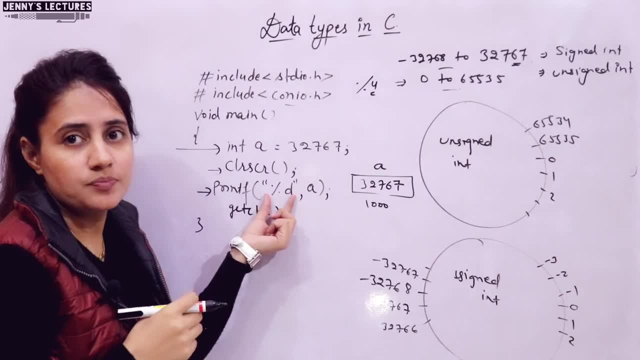 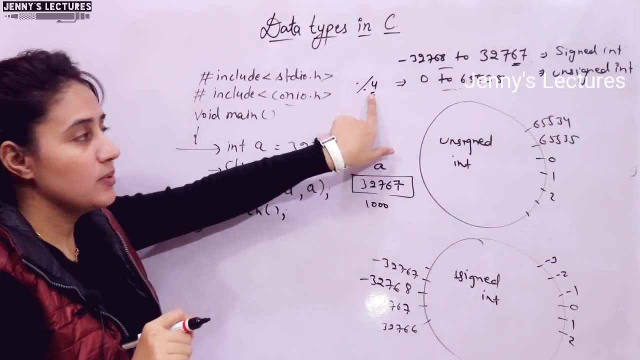 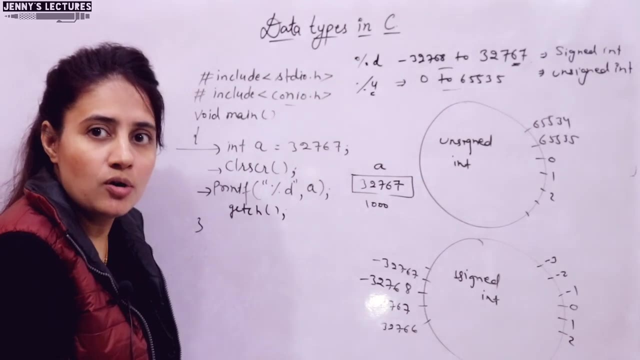 only %d means you are going to print integer value, Integer, and you can say that signed integer value, because for unsigned we are taking format specifier %u. For this one signed, we are taking %d and for short integer also you can use this one, %d or %hd, Both are correct. 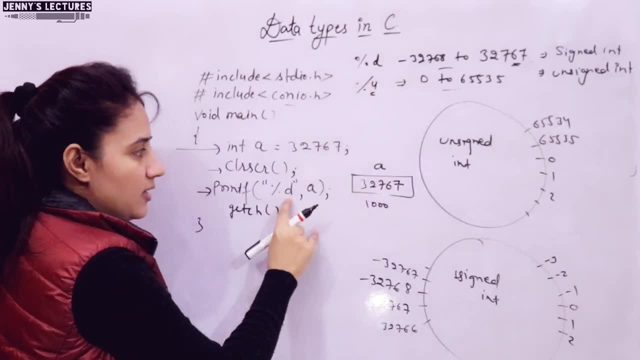 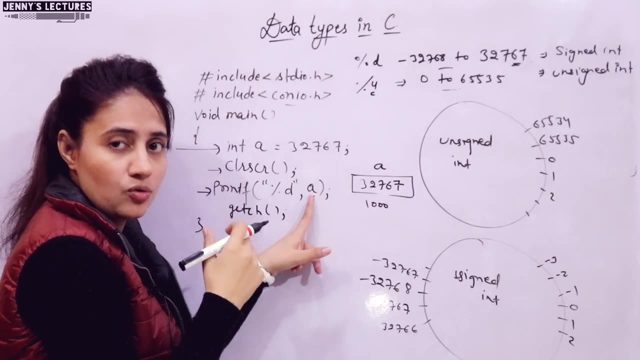 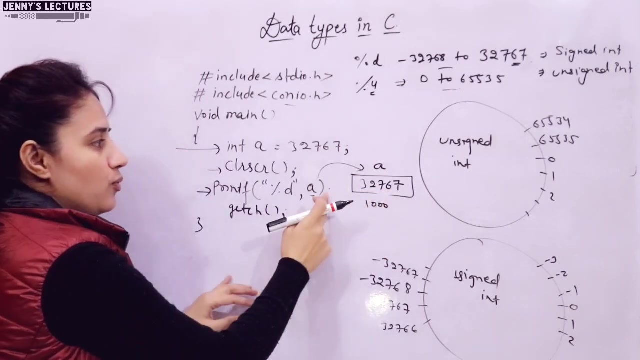 Right For unsigned. it is %u, So it is for signed integer Right Now. next value is what is a? So from where the compiler, the control, will fetch that data from this memory location, and at this memory location we have 32767.. So the output would be this one, only 32767. 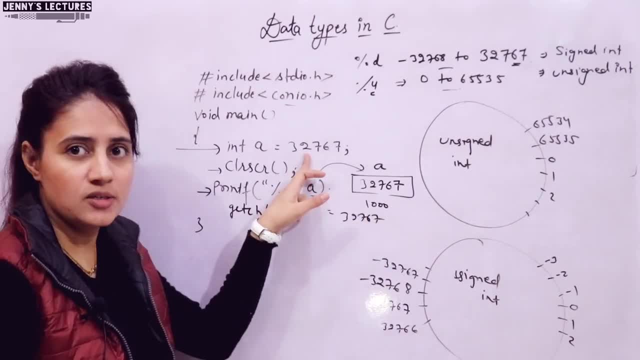 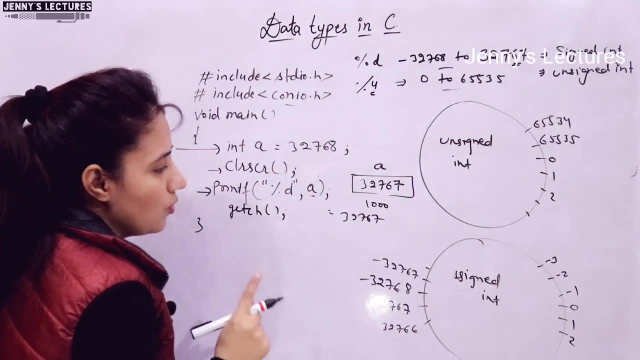 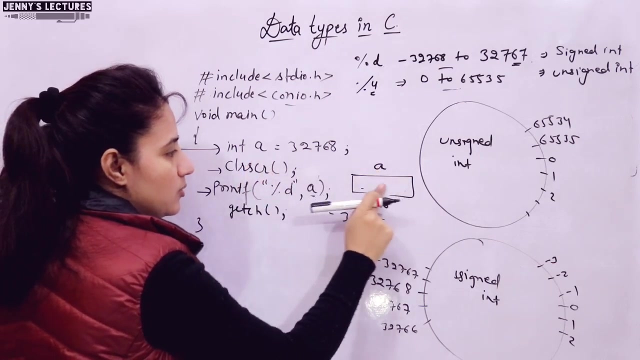 Right, You are getting same output. You are initializing this one and you are getting same output. Now let us take a different case. If I am writing here, 32768.. Now what will happen? See, it is signed integer. So this has been the data has been memory has been initialized. 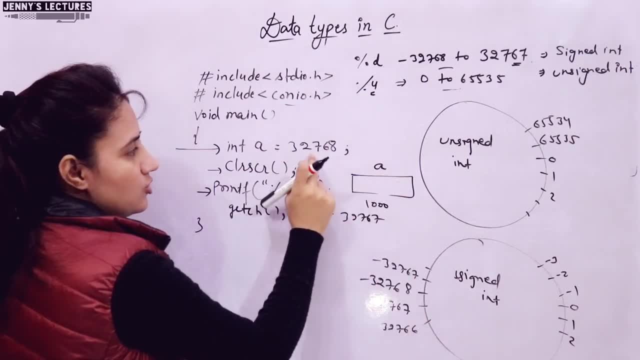 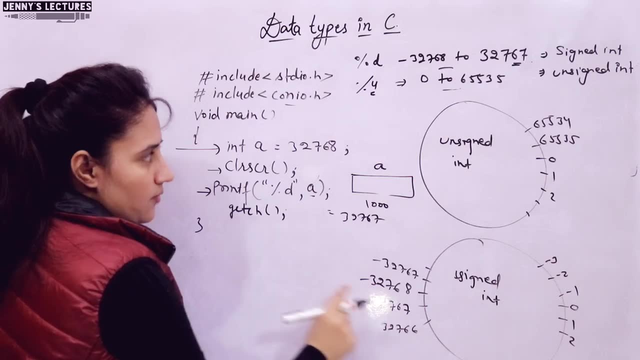 to a. So according to signed integer, see this: 32768.. Check out it is within range or not. The range is up to 32767.. Since we are going to add one here and here, its is out of range. but it will not give you. 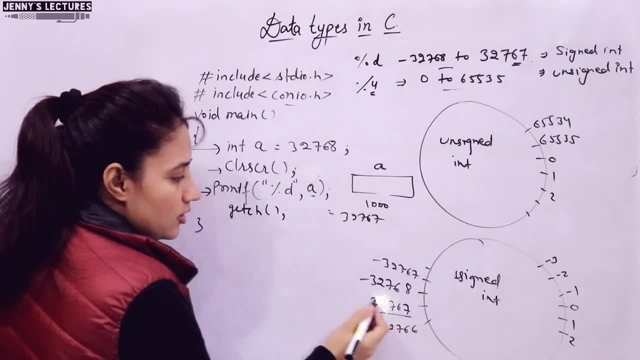 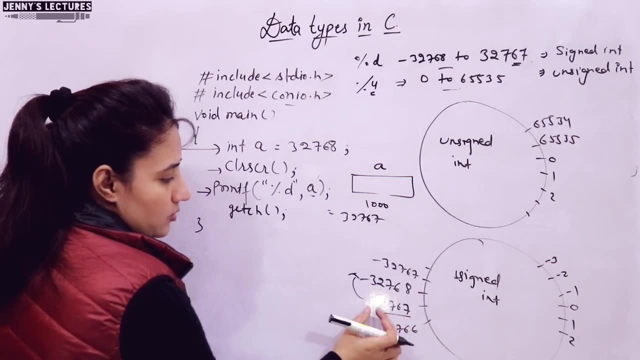 error Right, Because it will initialize here what value after this one we have, what minus 32768.. So if we increase one like 32767 and this is what 32768 according to our circle, So this value would be a signed minus 32768 would be a signed to this a. 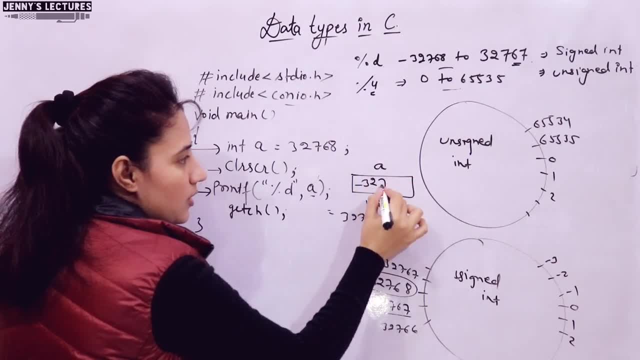 So now, when you will actually take the多少 menos or minus two of ApiA, Is pmc its absolute average value? Of course it is not our K files. a, The value is 0.05 into K обрат. instead I should have set a below k as minus k, and that is because k number is left over k, So 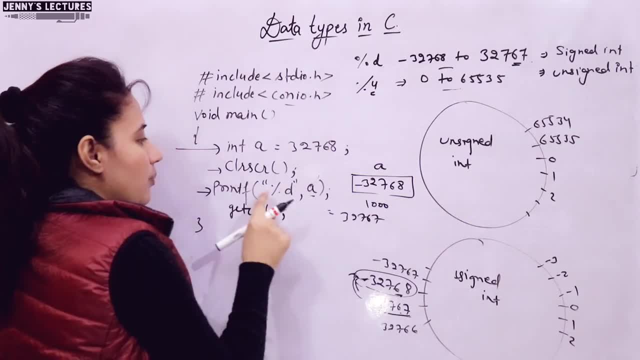 without komado p, and instead I will try to do something by relieving. what value will this be? times u, which will be 0. I got off the lowercase letter, which has purpose, it will be وه. So now, when you will print this one, what value would be printed? 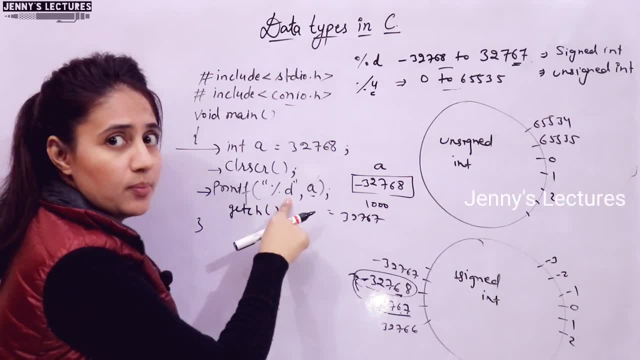 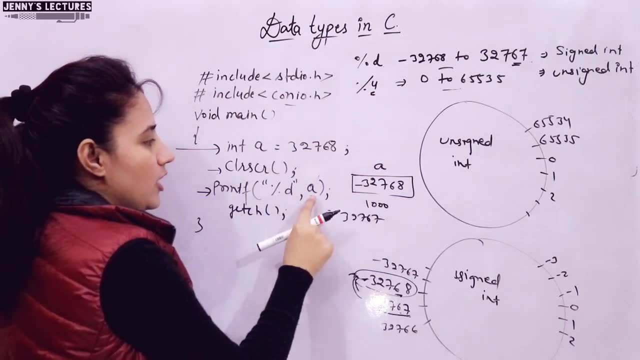 See when you will print like percentage D means you are printing what Signed int. For unsigned we will use percentage U. So here the value of A. what would be the output? This you will get output Minus 3,, 2,, 7,, 6,, 8.. 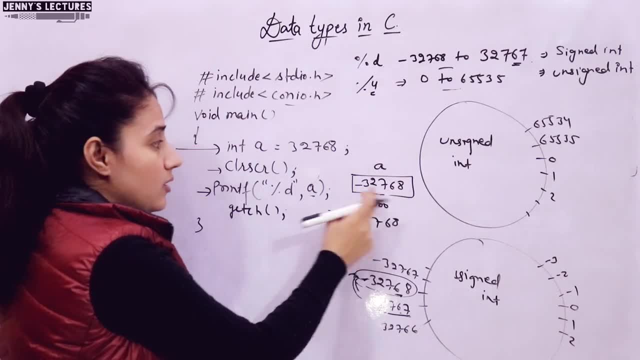 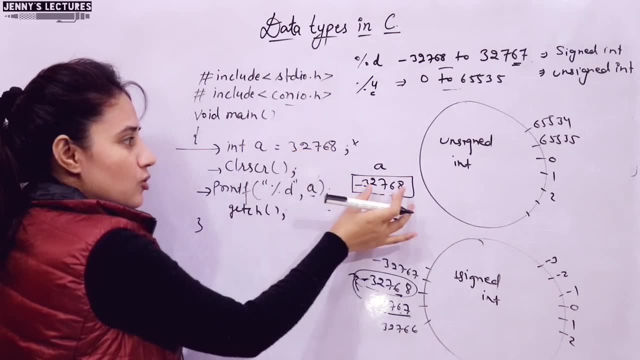 Because in memory this has been stored Right. The output will not be taken from this line. Because the function of this line is what? Just to allocate memory to this variable and store whatever you have given, But the stored value is this one. 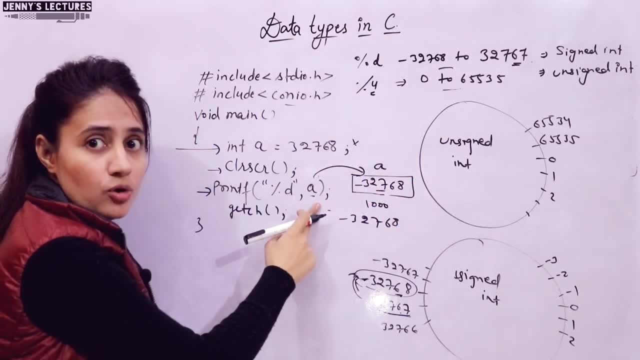 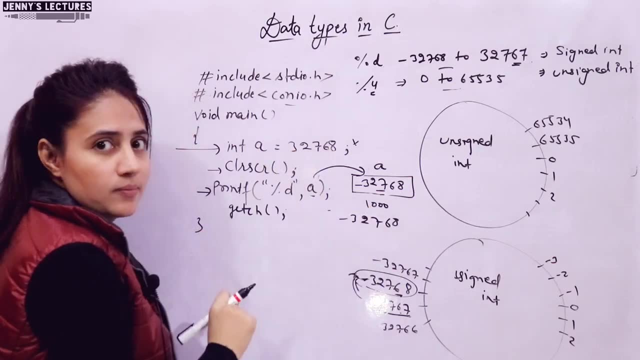 So from memory it is going to fetch. So from here it is going to fetch. Now, output would be minus 3, 2, 7, 6, 8.. But you have initialized this one, So this is what you can say. 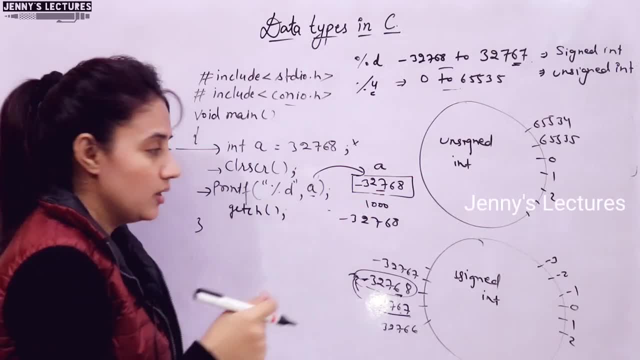 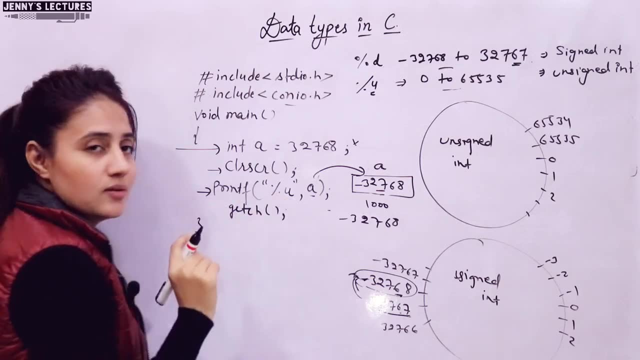 For you it is some garbage value. It is not correct. But it is not giving you error. And suppose if you will print here percentage, U, U and A, So this is what U is for unsigned integer. So check to this circle. 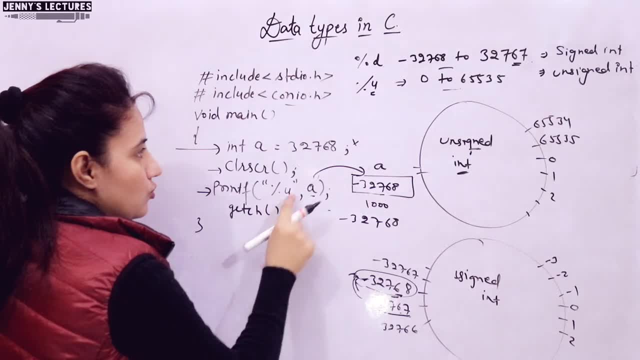 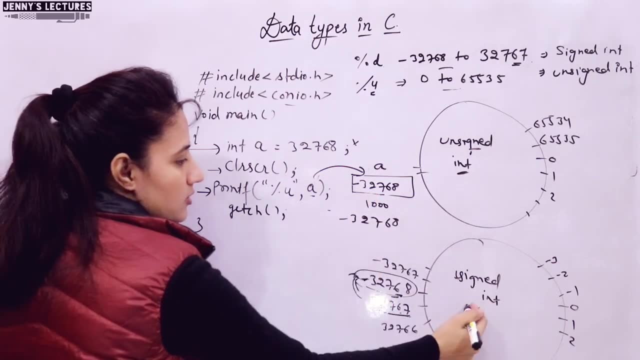 That is unsigned integer. Now here while printing percentage U. The value would be assigned, this one only, Because it is what Signed Here. we have signed integer, So this value would be assigned. It will check this circle. Now here. percentage U. 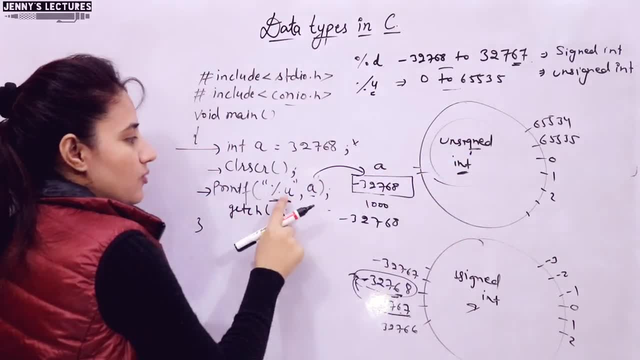 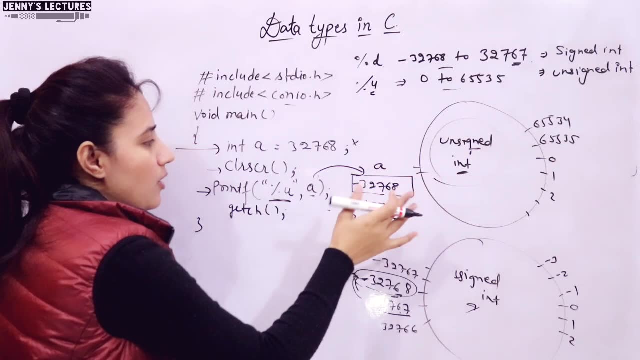 So it is for unsigned int. So now check while printing The format specifier: is this one, And this is very important. So now we will check while printing This value Right. So now check Here: we have minus this value or not? 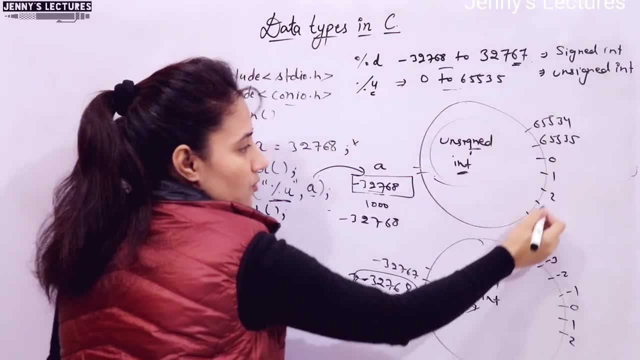 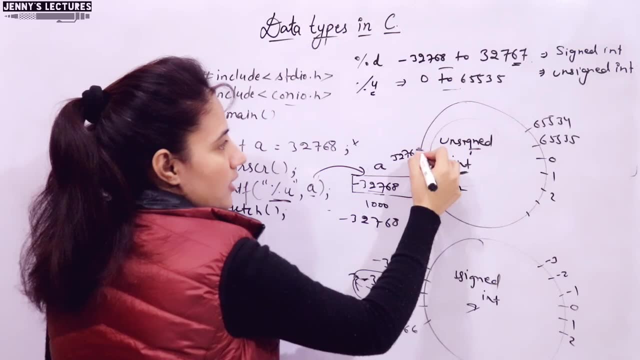 Here we don't have any minus sign, But you can say somewhere: Their value would be like 3,, 2,, 7,, 6,, 7.. 3,, 2,, 7,, 6, 8.. 3, 2,, 7,, 6,, 9.. 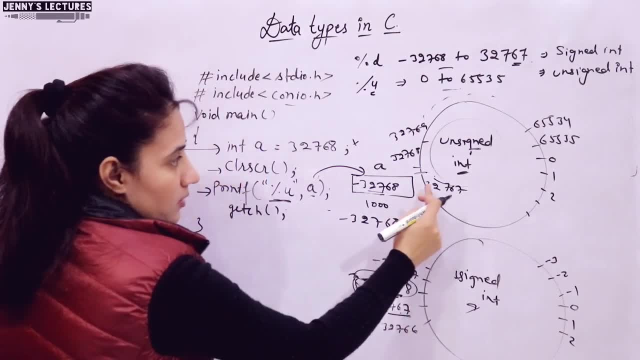 And up to we have this value. So now check this one: 3, 2,, 7,, 6, 7.. And here we have 3, 2,, 7,, 6, 8.. Minus 3, 2,, 7,, 6, 8.. 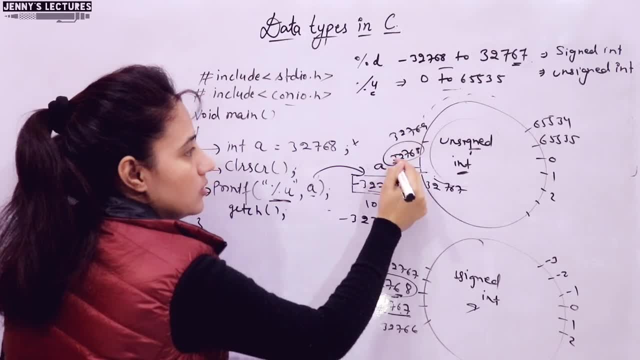 But corresponding to minus. Here we have what Positive value? only 3,, 2,, 7,, 6, 8.. So here it will give 3,, 2,, 7,, 6, 8 answer, Not minus value. 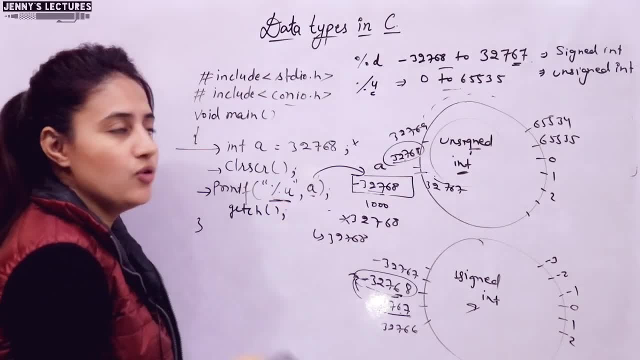 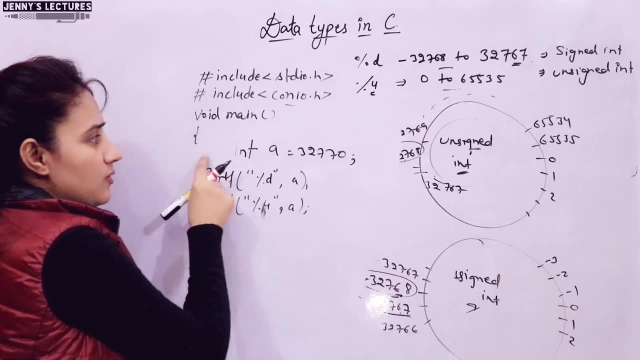 Because format specifier is percentage U. If you will not get this one, Let me take one another example. Let us suppose you want to store 3, 2, 7, 7, 0.. This is what I am not writing, anything. 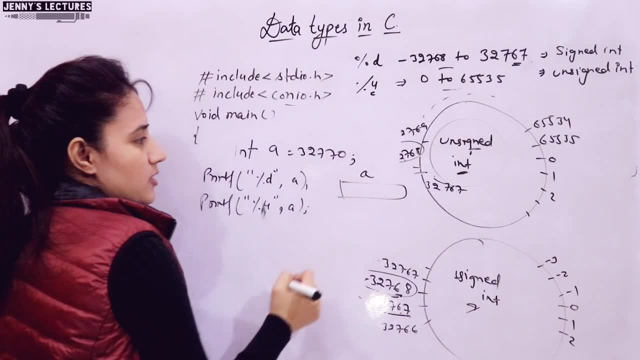 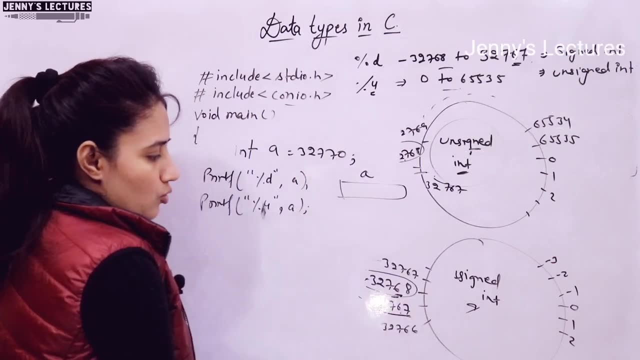 So this is signed integer. So now in a memory Space has been allocated to this A. Now check in signed integer. Do you have this value: 3, 2, 7, 7, 0.. No, This is out of range. 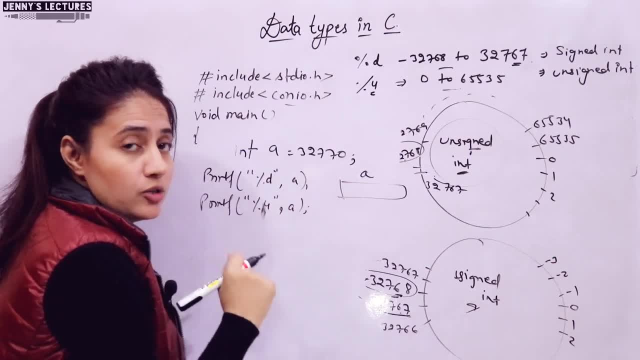 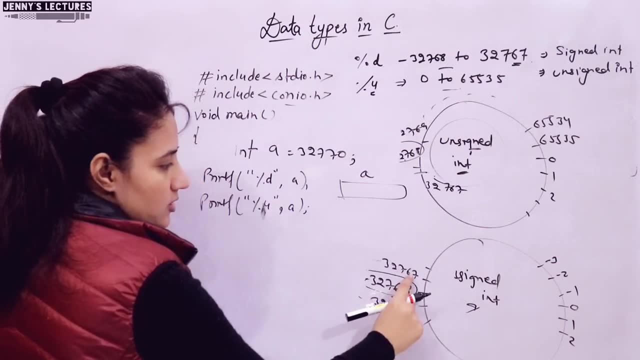 But it will not give you error. It will put something in this memory, But what it will store here? See up to this one, we have 7, 6, 7.. This is 7, 6, 8.. 7, 6, 9.. 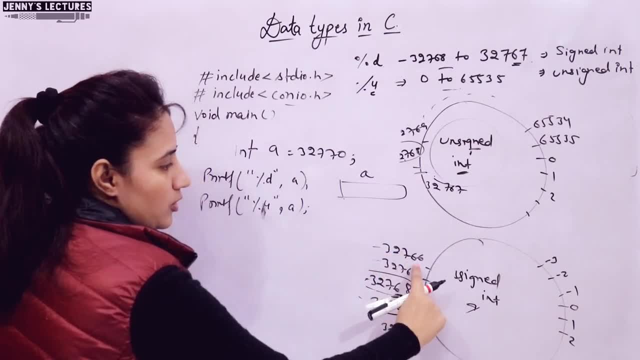 And minus 3,, 2,, 7,, 6, 6.. This is corresponding to 7, 7, 0. So this value would be stored Minus 3, 2,, 7,, 6, 6.. 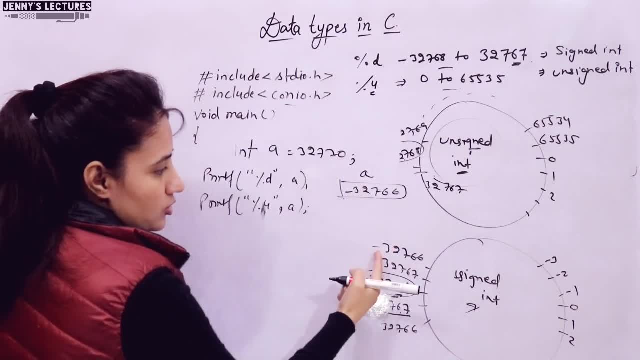 Right: 67,, 68,, 69,, 70., 70. So this minus, But sign is minus in this circle Because this value is not in this range. So this would be Stored When you will print with percentage D. 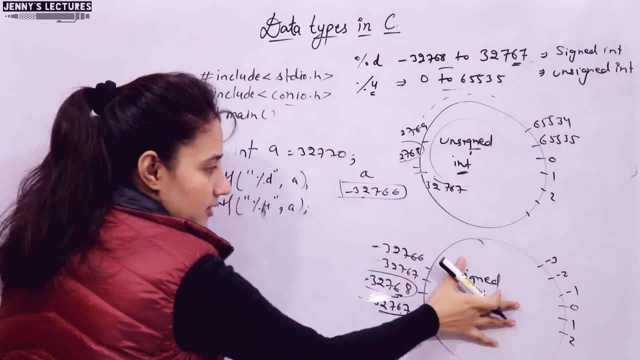 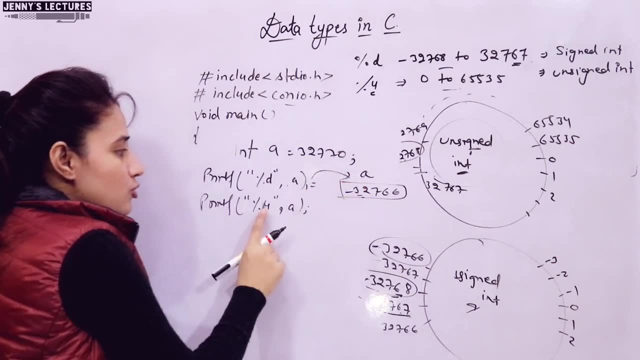 Then percentage D means Signed integer In signed integer. Do we have this value? Yes, we have this value, So it will fetch directly this value. So output of this line would be this one. But suppose if you are printing it with percentage U? 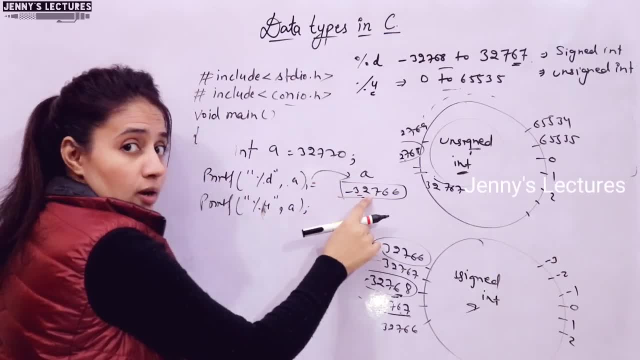 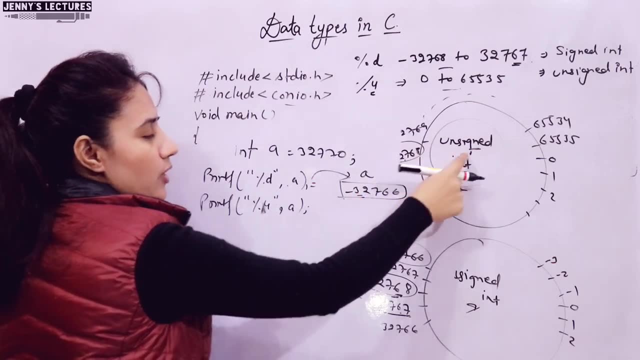 That is unsigned integer. So now, value would be stored, this one, But while accessing the value, It is percentage U It means unsigned integer. It will follow this circle. Do we have this value in this circle? What is the value Corresponding to this one? 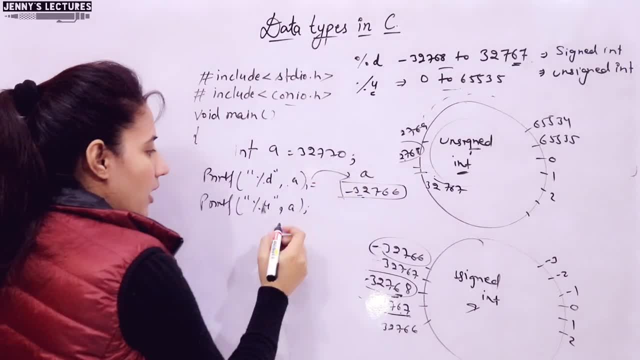 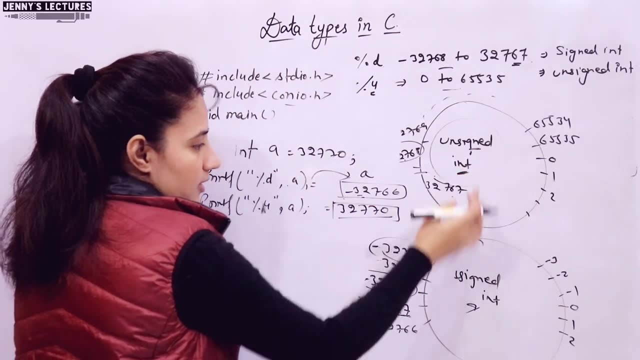 We don't have minus sign, So corresponding to this, In this circle We have only 3,, 2, 7, 7, 0 only. So it would be printed for percentage U Right, Because see this circle and this circle is almost same. 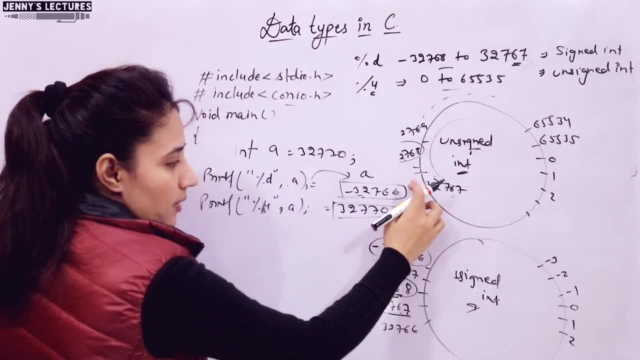 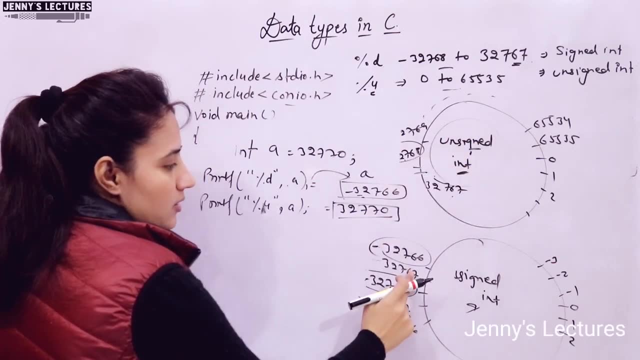 You can check out here: up to 67. Here would be the same number, and after 67,, 68. But sign would be positive only because it is unsigned. Then 69,, then 70. So corresponding to this in this one, here we will have 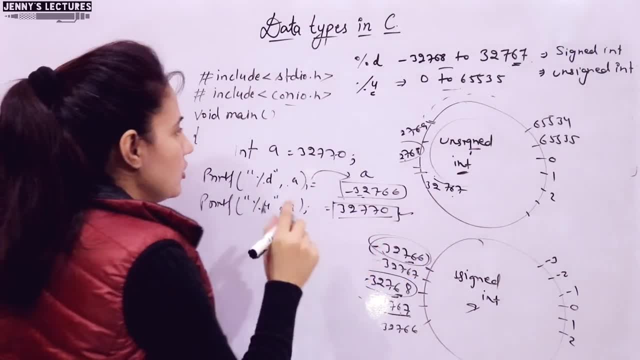 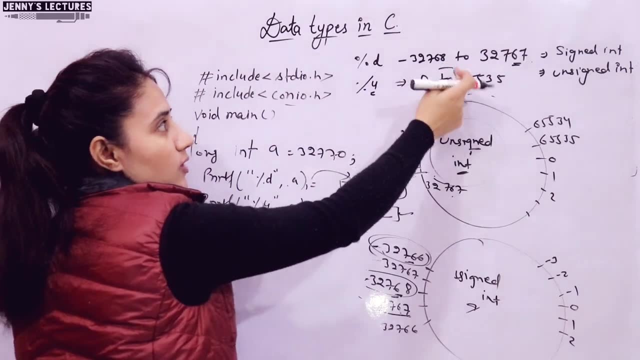 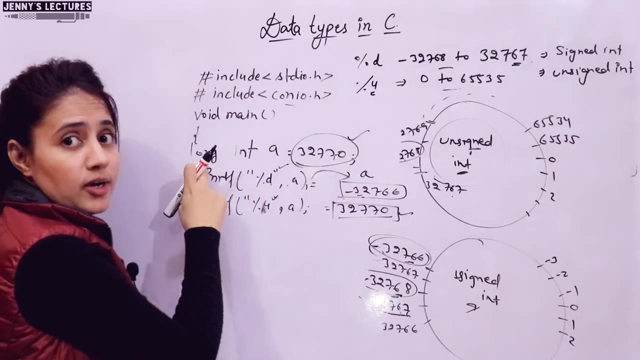 70 only. So it will print 70. Right, But suppose if you are taking here long int, So the range of long int is what It's. beyond that, this range. In the previous video you can check out the table. So this would be within the range because we are taking long int. 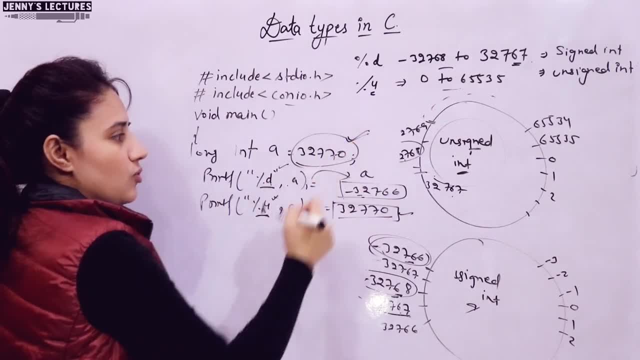 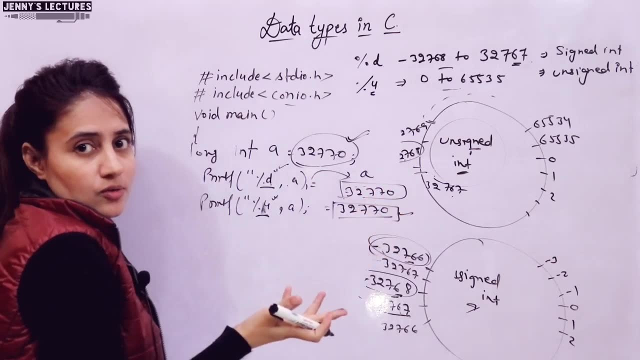 So both in case of percentage D and percentage U, it will print this only Because number would be stored as it is 3, 2, 7, 7, 0.. Because of that range, we are having this number within. 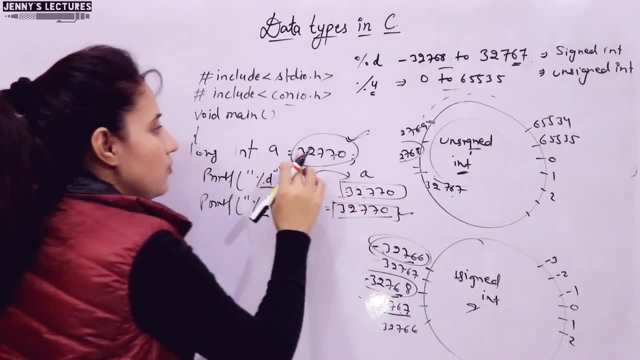 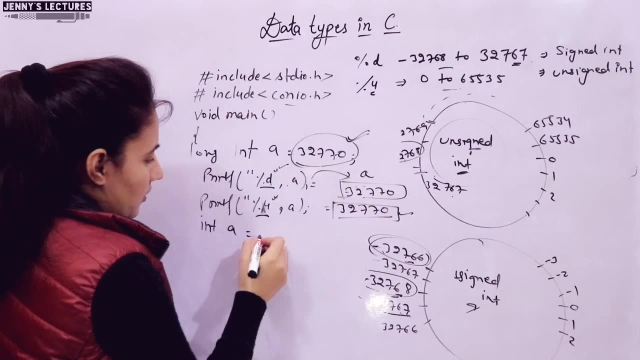 The range. So that would be same output. Suppose if here I am taking int A 655.. Not 655, I am taking, suppose, minus 10. And then I am printing with percentage D and percentage U, Then what should be the output? 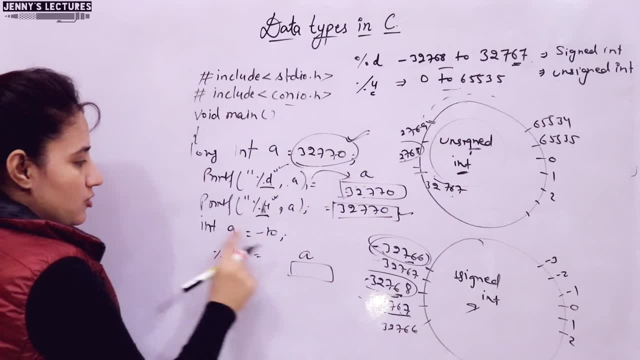 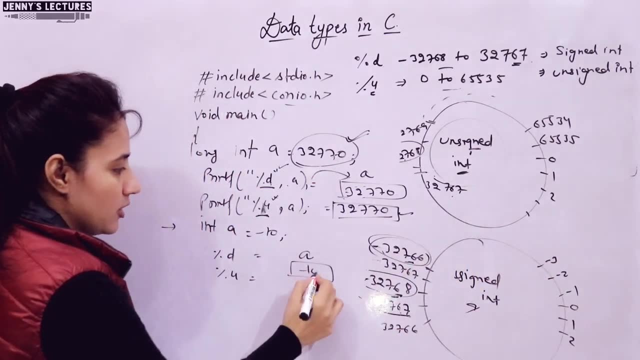 What would be stored here in A A is minus 10.. It is signed integer In signed integer. do you have minus 10?? Yes, we have minus 10, because both minus plus value we have. So minus 10 would be stored. 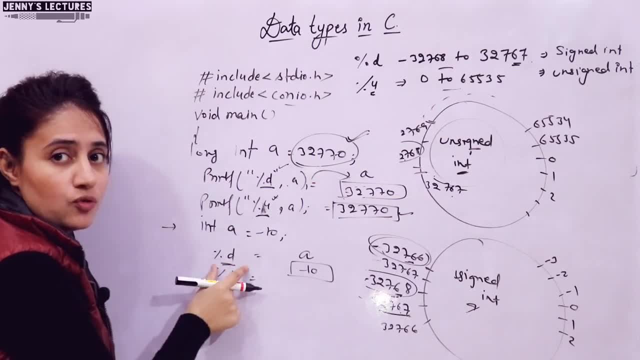 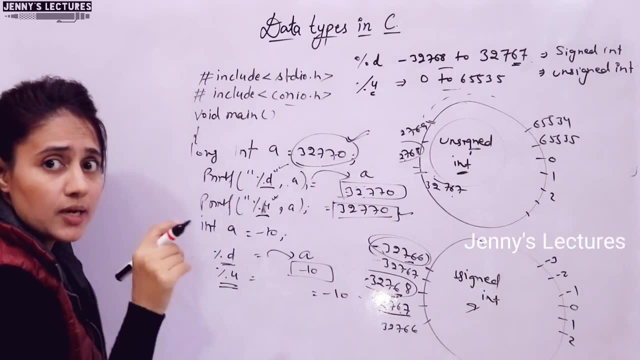 When we will print with format specifier percentage D, it means it is for signed integer. definitely it is going to print minus 10.. When we will print with percentage U, this format specifier is what It is going to print: unsigned value. but this is signed. 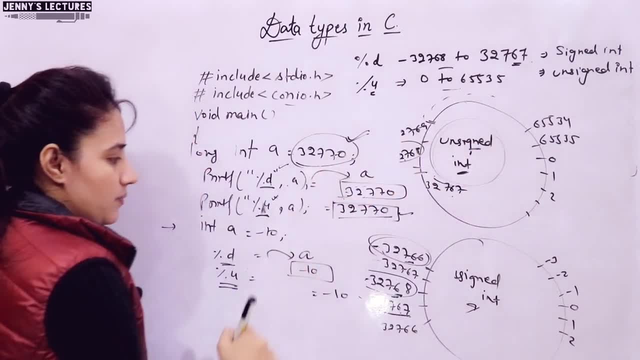 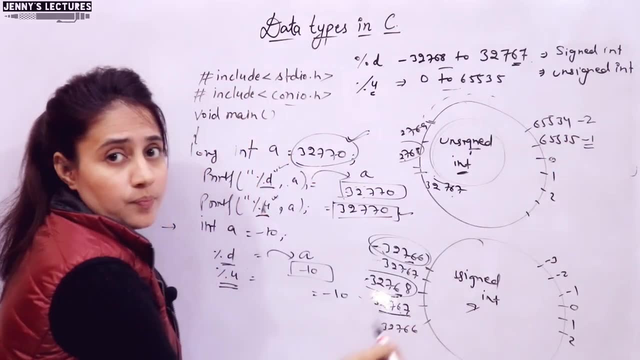 So corresponding to this, what is value in this unsigned circle in minus 10?? If we go reverse, then it is corresponding to minus 1, it is corresponding to minus 2.. Like this, the value corresponding to minus 10.. That would be printed. 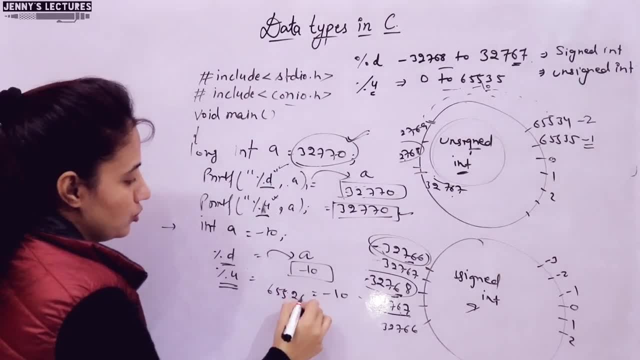 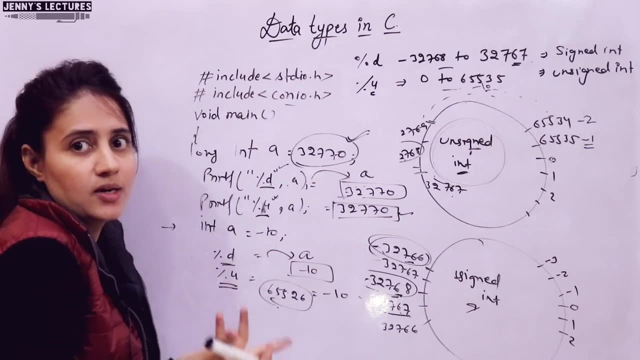 And that value is what? 65526.. So you are initializing minus 10, but you are getting answer this one. That is why the reason you are getting different answer may be: But suppose in long int I am printing this number 7777.. 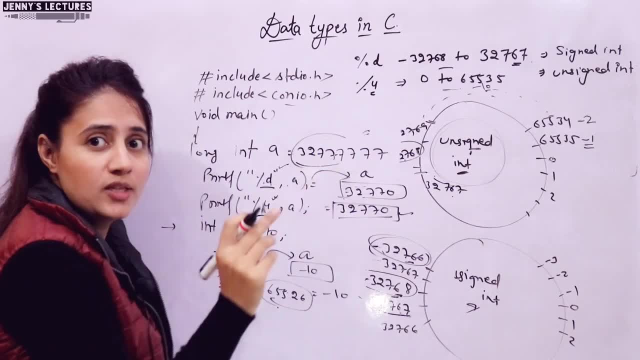 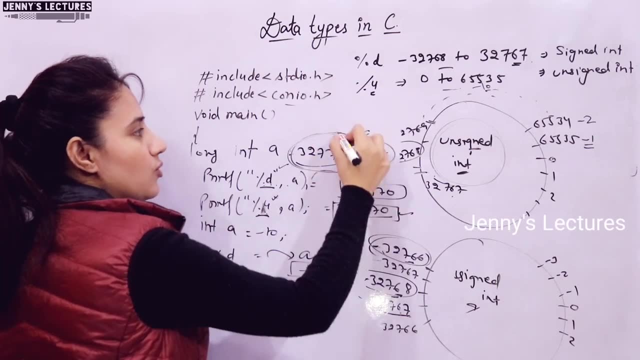 So what would be the output? We are using long and this number is within the range Right, So the same output would be printed: percentage D, percentage U: it will print this number only Right. And if you initialize, suppose int A is equal to 0.. 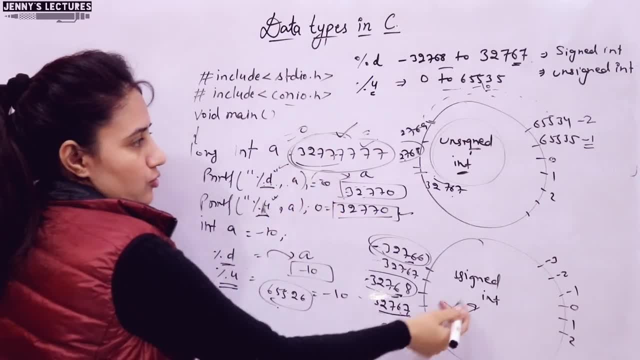 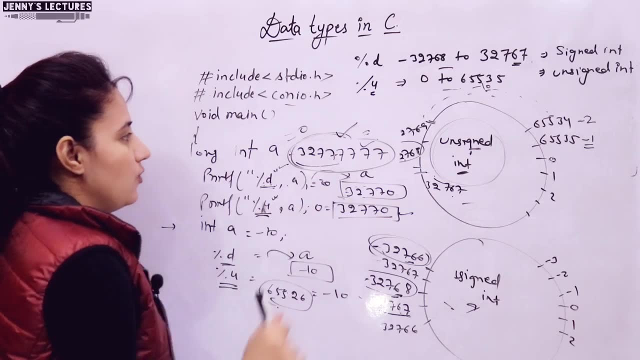 Then both will print here and here both will print 0 and 0.. Here also we have 0, here also we have 0.. Right, Both in signed and unsigned. So whether you will print with this format specifier or this, it will give you 0.. 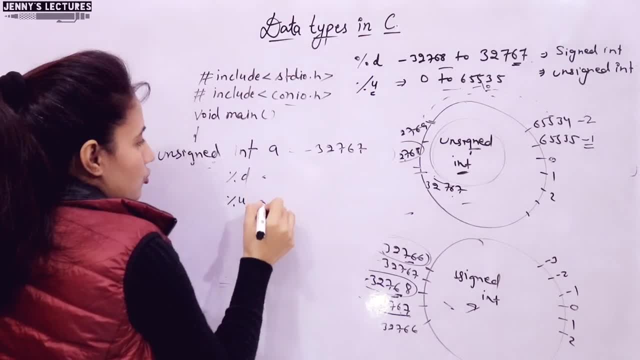 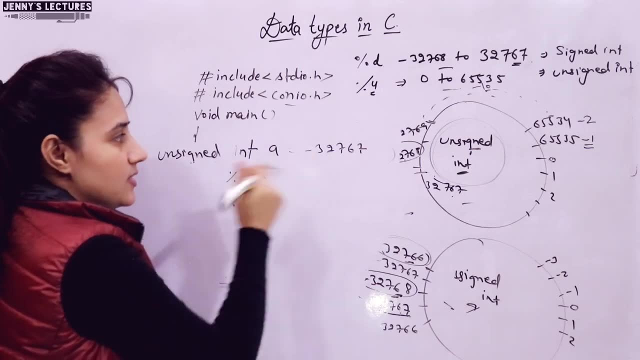 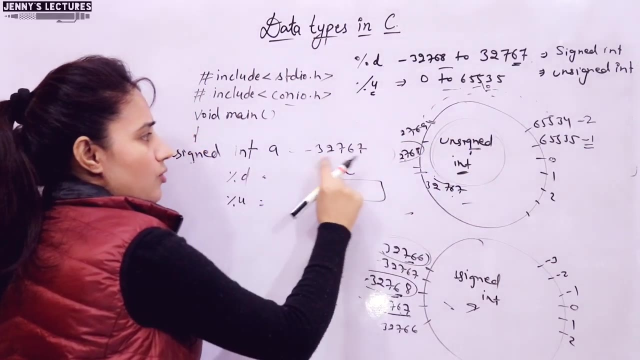 And if suppose you specify here unsigned int? So now you are specifying particularly unsigned int and you are storing minus sign that is signed, That this is a signed number. So now memory would be allocated to A, And what number would be stored here in unsigned integer? check out this one corresponding to this value. 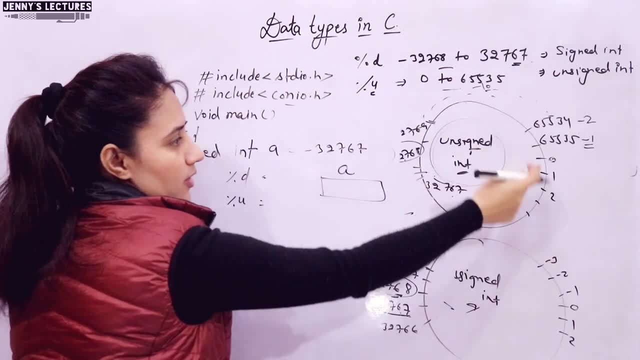 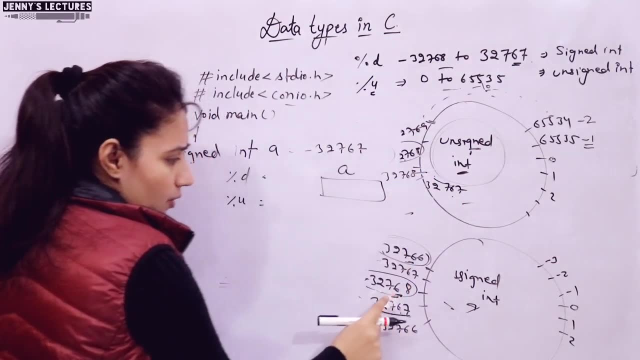 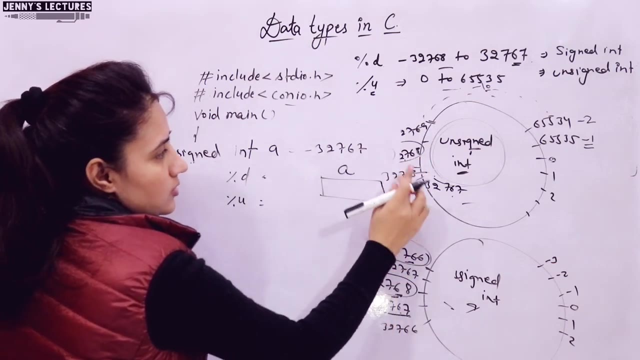 What should be the value minus 32767.. Here, somewhere we have 32767, then 32768, right Now. according to that, here we have minus 32767. now, corresponding to this value. what should be the value in this unsigned circle? It's 32769.. 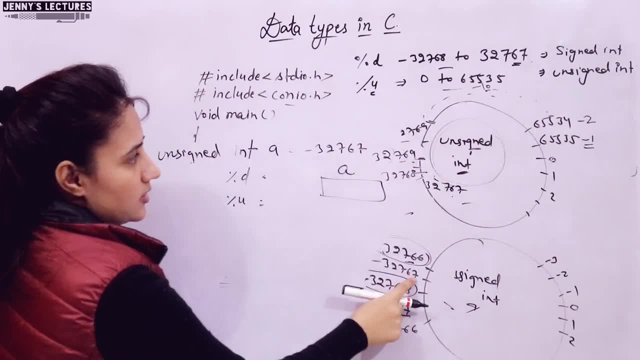 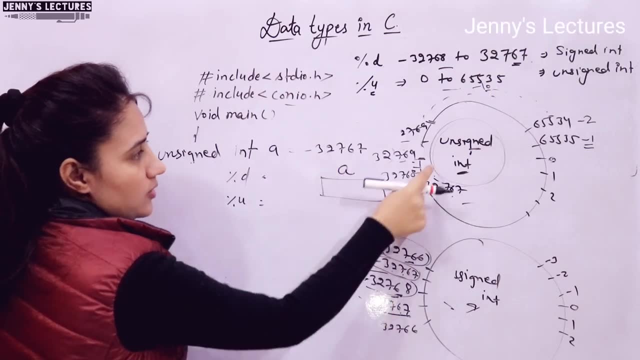 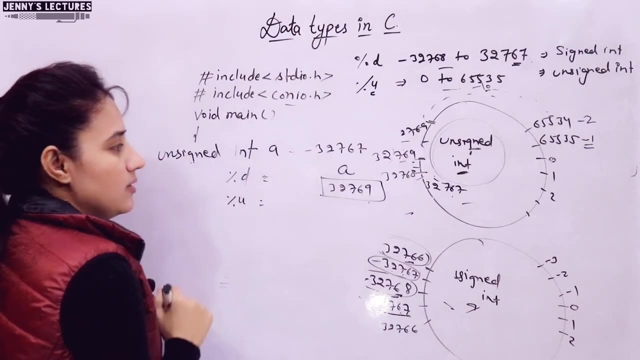 Right, Because here 767, 6869 right, And this is what exactly? minus 32767. this one is minus 32767.. So in this circle corresponding to this, we will get 32769. this value would be assigned Right Now when you will print with %d means %d signed integer. 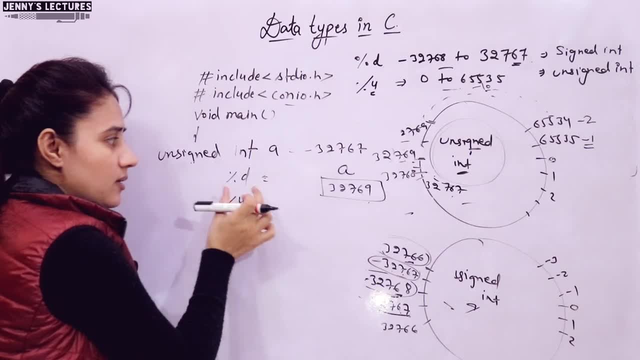 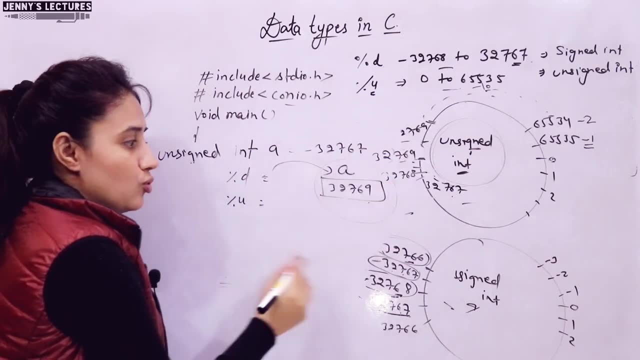 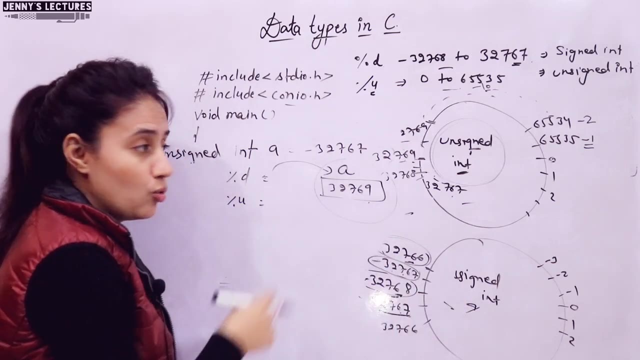 Now check this value is while printing. it is for signed integer, So while printing we are fetching from this from here, from memory also Only. So now refer. it will refer signed integer circle. So check this value is within this integer or not. This is not so corresponding to this value. what is the value here? 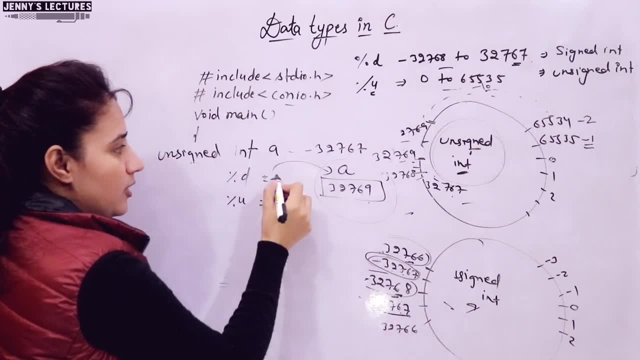 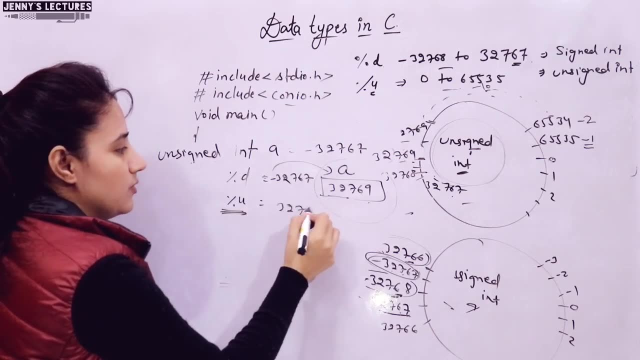 67, 6869 this value. So here it will print minus 32767.. And if you will print with %u, it will print this value 32769.. Because while printing with %u, it will refer to this circle, and in this circle do we have this value. 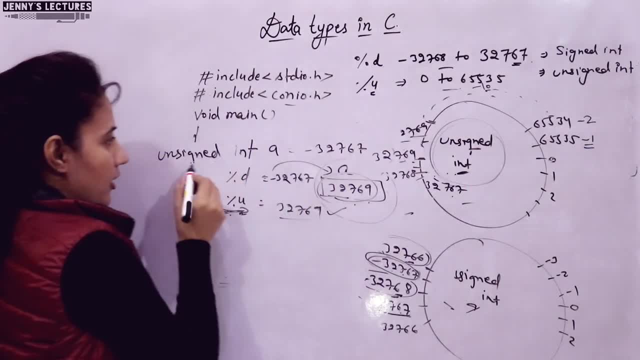 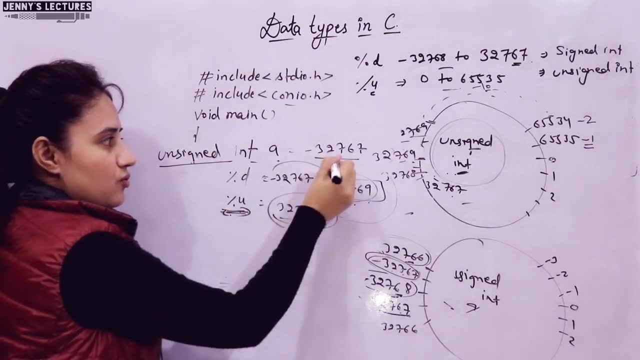 Yes, we will have this value, so it will print this one right? So see, here you are assigning unsigned int this value, but when you are printing with unsigned number, then you are getting different answer from the initialization value. Because the range? because of the range. 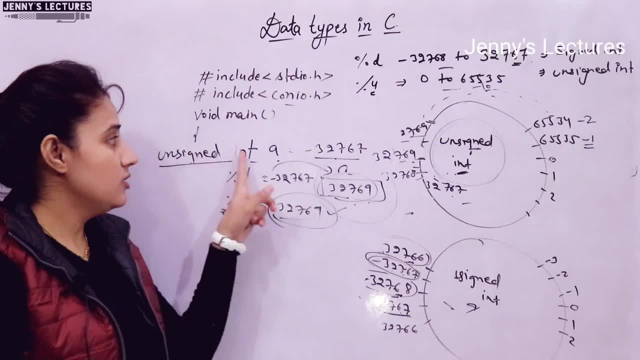 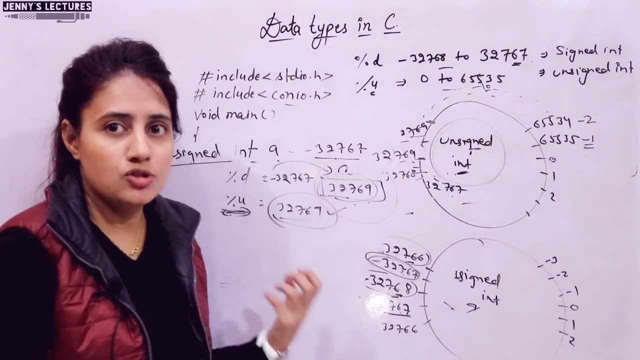 Right. According to that, you can check out the short integer range also, and according to that, you can check out the long integer range also. You just have to practice this thing. It's not like that, Just watching YouTube videos And just by seeing these lectures, yeah, you got it. 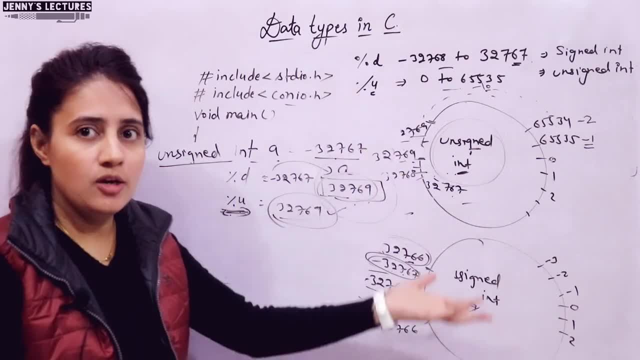 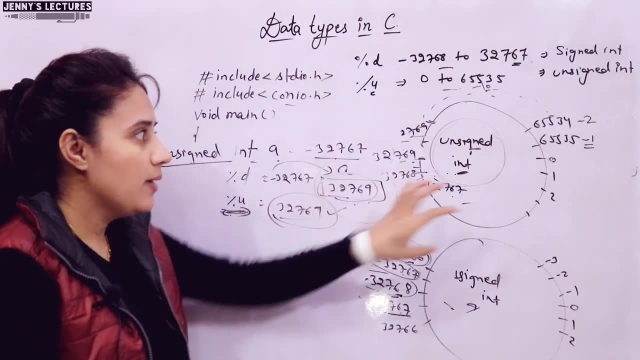 No, you have to practice with your own hand. Try to initialize different, different values and try to find out what should be the answer Before getting answer on your system. Brydon that program with these two circles- signed int, unsigned int- and find out output with your own hand. 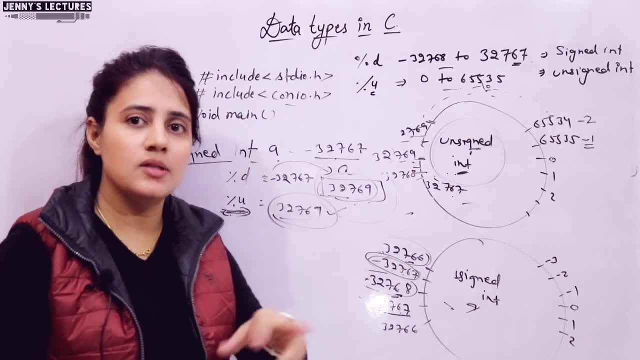 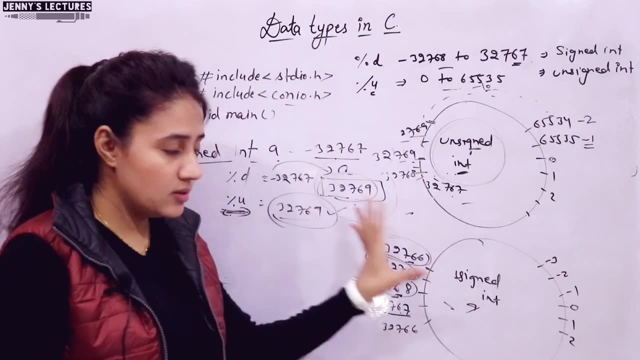 Then check with your system, then compile and run and then check with your system and tell your answer is correct or not Right? So maybe next video we'll discuss about care, Everything we have discussed about in that thing. we'll discuss about character, with some examples. Right, So now I'll see you in the next video. till then, bye, bye, Take care. 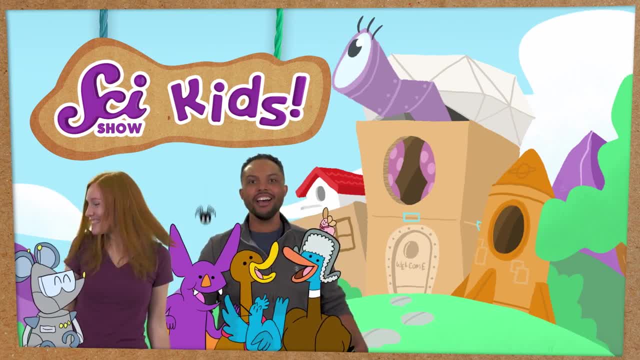 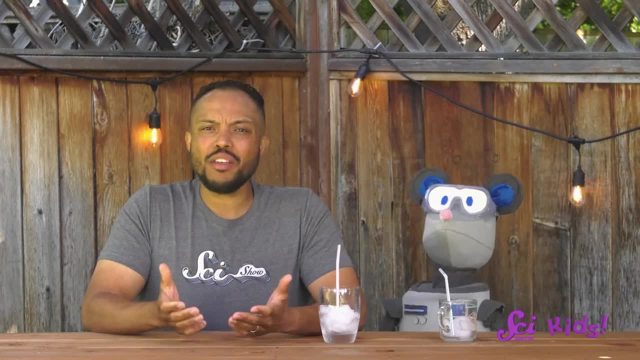 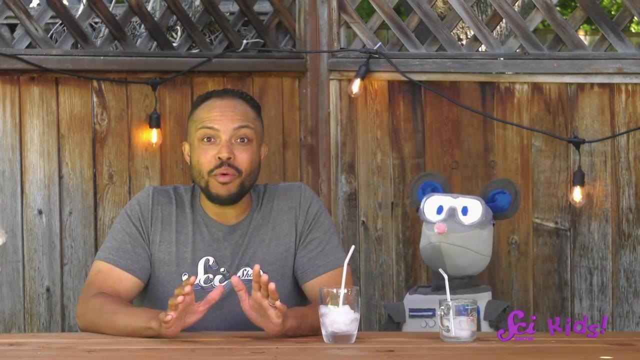 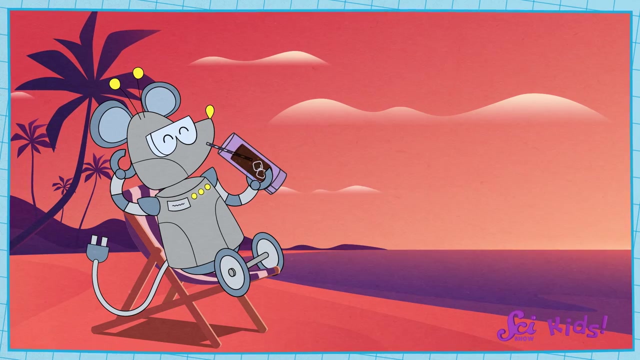 That was refreshing. There's nothing like a nice, cool drink on a hot day. What's your favorite refreshing drink? Squeaks, I love that one too. My favorite is strawberry lemonade. Sometimes Squeaks and I even have some soda as a treat. We love the tingly feeling. Great question. That tingly feeling actually comes from lots of tiny bubbles. People that make soda squirt the bubbles very quickly into the soda and then put a cap on the bottle so the bubbles don't escape. We can't see all the bubbles, but they're inside the bottle with the soda.